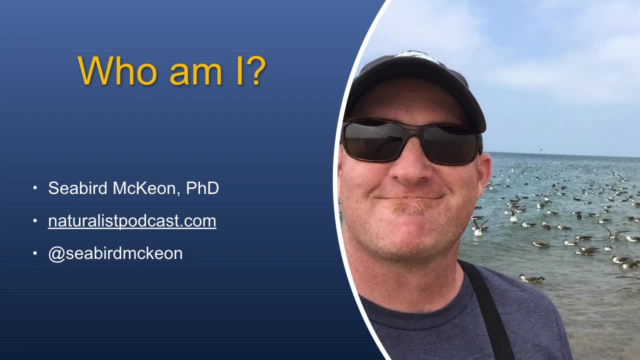 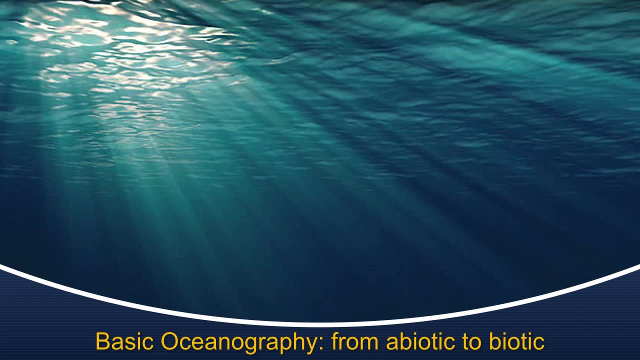 of different other places. In our last lecture I talked about how the chemical and physical properties of water are important for life on Earth. In this lecture I want to try to use basic oceanography to take us from the abiotic factors that influence the marine 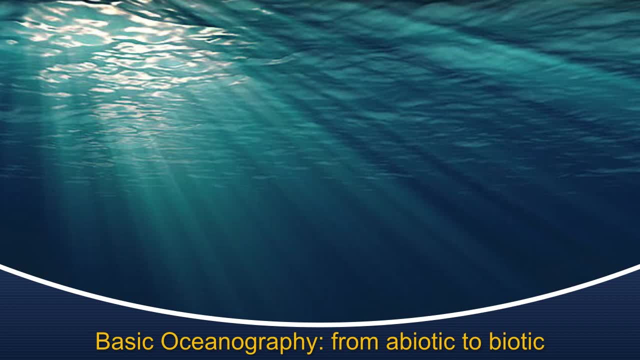 environments into the subject that really brings us all here, which is marine biology. Oceanography is a huge topic in the marine biology field. It is a huge topic in the marine biology field in its own right, and to do it justice will take more information than 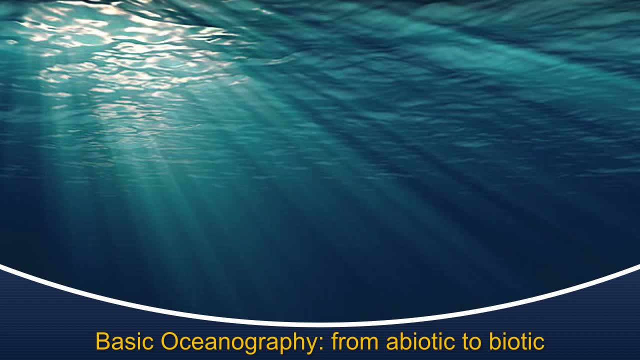 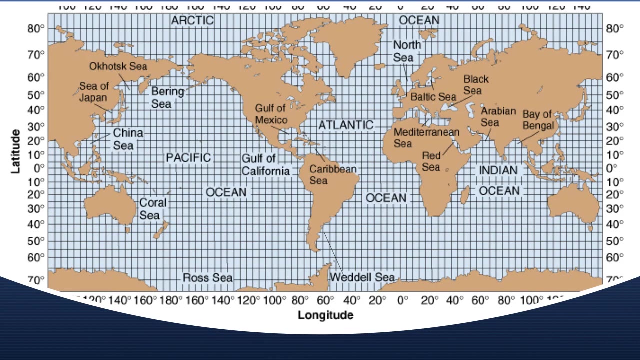 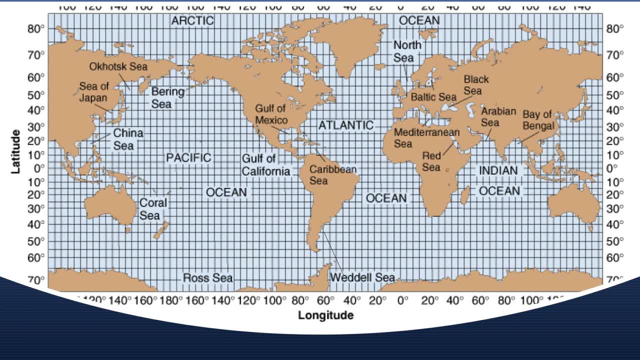 oceanography. All of this is a map of our planet that we, as humans, will know when we overcome the uncertainty and fear. but all of this stuff has led me to see something that we don't know but think about. Okay, so what is the river? we assume a specific origin, for It's useless to ask for information. 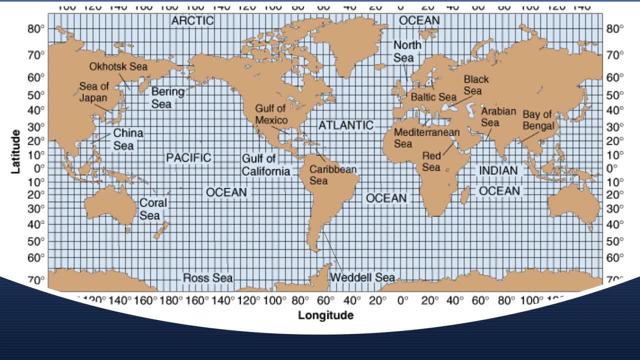 at a recent hagoand we have the water of the ocean. Let's take this that we didn't know, not just seven of them. So we've got the Mediterranean and the Caribbean, the Baltic, the Bering, South China, coral, Oktausk- all sorts of different seas, But it's important to remember. 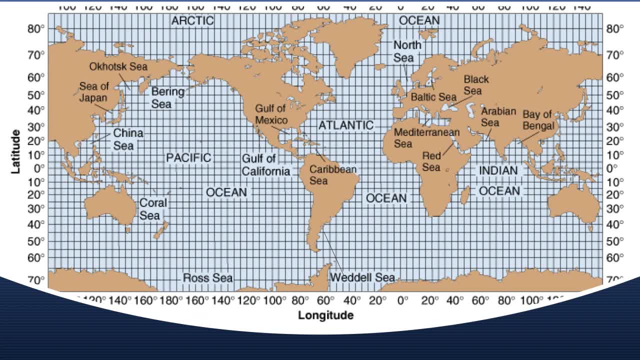 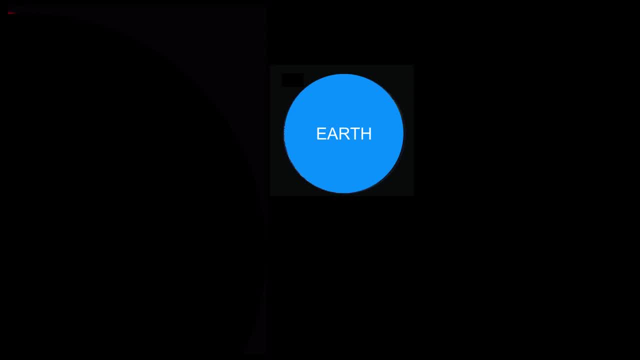 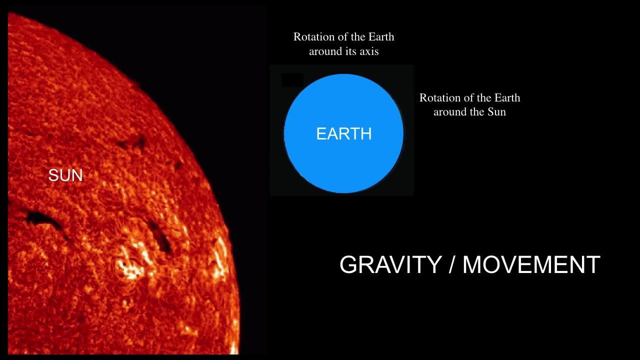 that all of these bodies of water are connected, And they're connected enough that our planet appears mostly blue from space, And our pale blue dot in space has a few abiotic influences. We'll start with gravity and movement. The formation of the earth had a lot to do with gravity and movement, And these are the forces. 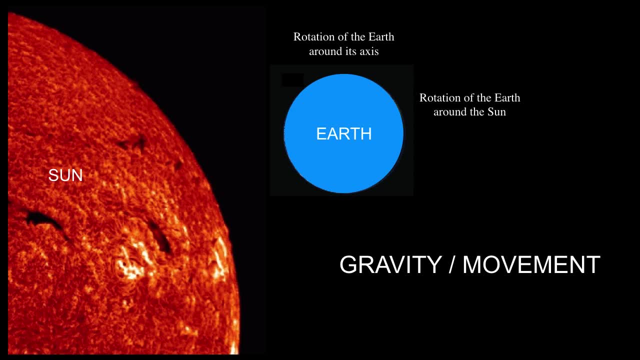 that still have tremendous influence on how earth works. So there's the rotation of the earth around its axis, the rotation of the earth around the sun, the rotation of the moon around the earth. so movement and gravity are still playing a large, large role in how our planet works. 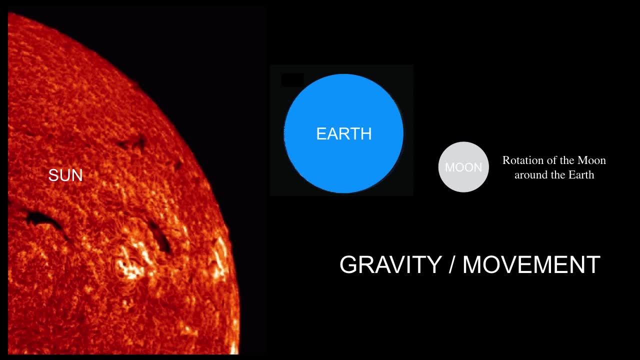 But the one that I think is most important for us to discuss right now is light. So the big one is light from the sun. So solar radiation from the sun heats the earth and creates the winds and drives ocean circulation, But it doesn't do this evenly So, just because of the tilt. 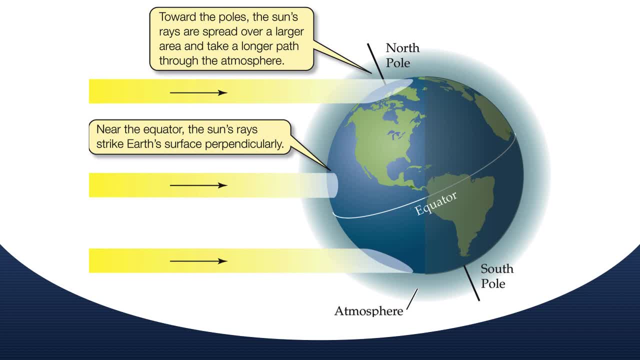 the amount of light that hits the earth coming from the sun varies depending on where you are on the earth. Right around the equator, the sun rays strike the earth almost perpendicularly, right straight on, Whereas if you're up towards the pole, the rays of the sun are spread out over. 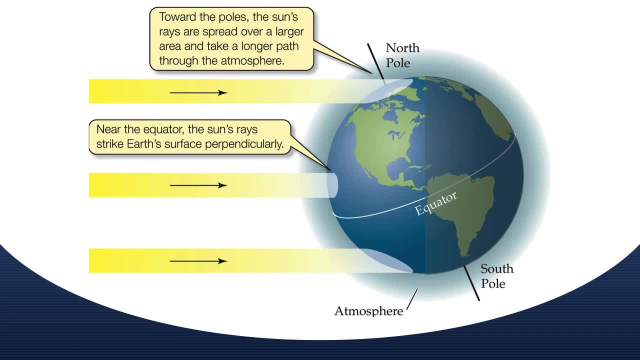 a larger area and take chance. So this isn't going to happen. This isn't going to be a very long or a very objective Ganod Slowly楽 Studio wasn't meant to generate information about Provost Frog's. take a longer path through the atmosphere. 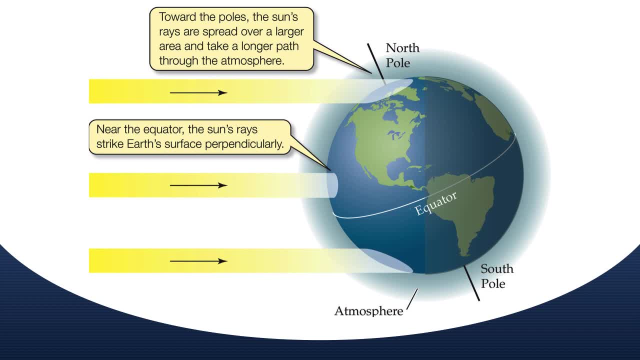 And this differential heating of the Earth's surface is why we have temperature differences on our planet. If the planet was completely water, we would expect to have some fairly even patterns, some seasonal variation, but it would be a smooth progression as we go from the equator. 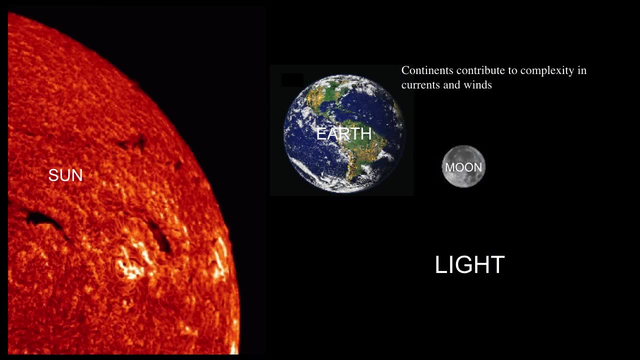 towards the North and South Poles. This is made more complex by the presence of the continents, So the continents. disrupting the flow of air and water masses over the surface of the planet really shakes things up a bit, changes the way that we expect this differential heating to impact the Earth. 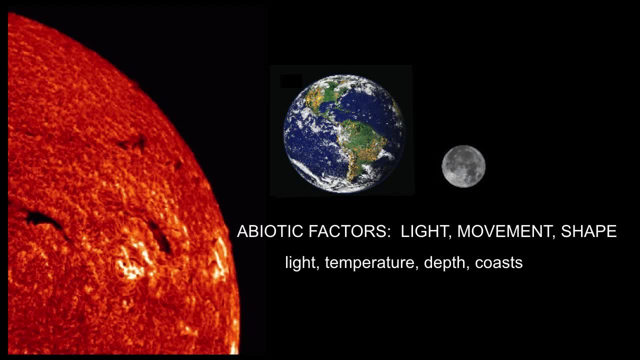 So when we're talking about abiotic factors, I really want to be focused on light, the movement of air and water masses, how those things are interacting with the shapes of the ocean basins and coastlines, And when it comes to light in particular. 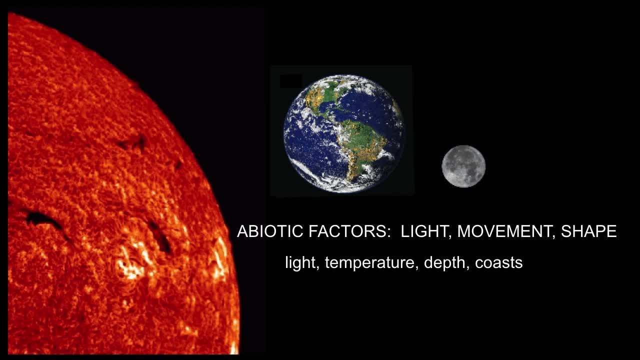 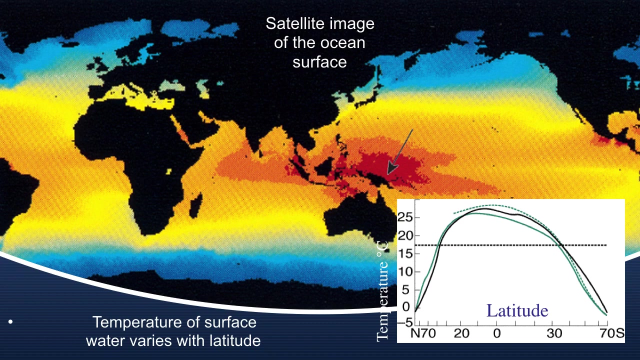 we're thinking about temperature. How is solar energy transferred into temperature of water And depth? Do we lose light as we get deeper? Yes, And those coastlines. how does it all interact there? So here's a satellite image of the surface of the ocean. 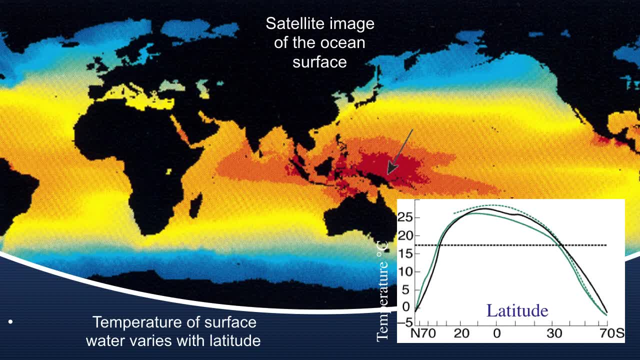 And the hotter colors- so reds and oranges are higher temperatures- The cooler colors- greens and blues- are cooler. I want you to think about the fact that most marine organisms are poikilothermic, or or cold-blooded, you could say. 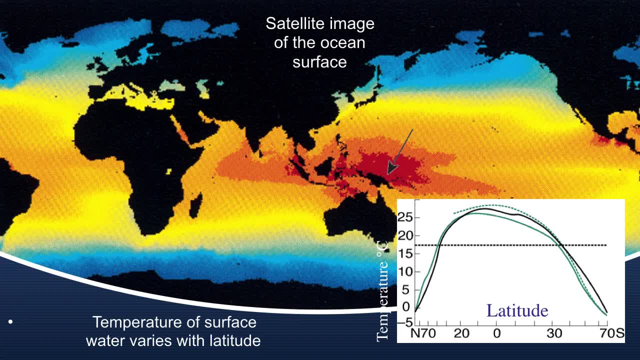 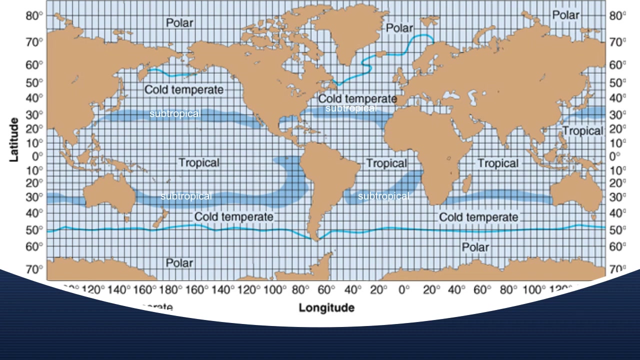 And since seawater temperatures vary latitudinally, the distribution of marine organisms is a reflection of the geographical differences in ocean temperatures And, based on surface ocean temperature and the distribution of organisms, we can start to describe four major geographic zones. So, starting from the north and working our way, 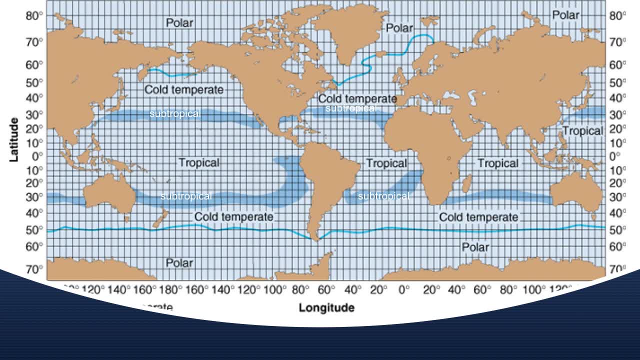 towards the equator. our major geographical zones in oceans, or at least the surface of the ocean, are the polar regions found at both the north and south poles of our planet. Then we get into what's called the cold temperate, right next to the subtropical waters. So we get into the cold temperate right next to the subtropical waters. So we get into the cold temperate right next to the subtropical waters. So we get into the cold temperate right next to the subtropical waters. 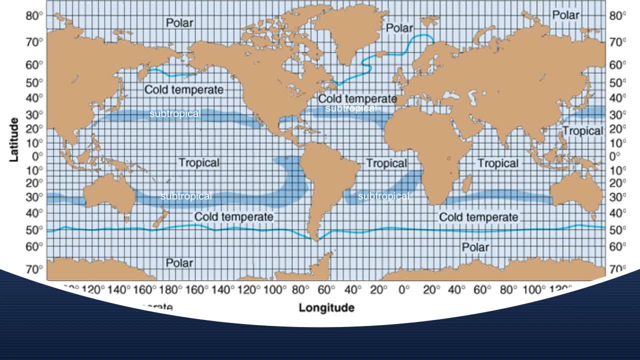 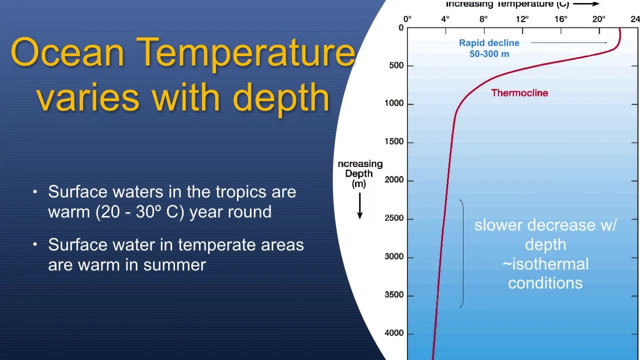 And this is where most of us have our experiences with the ocean. Tropical oceans are uniformly warm, and then the pattern repeats on our way south. So this pattern of four zones applies to the surface waters of the ocean, but it doesn't really apply to depth. 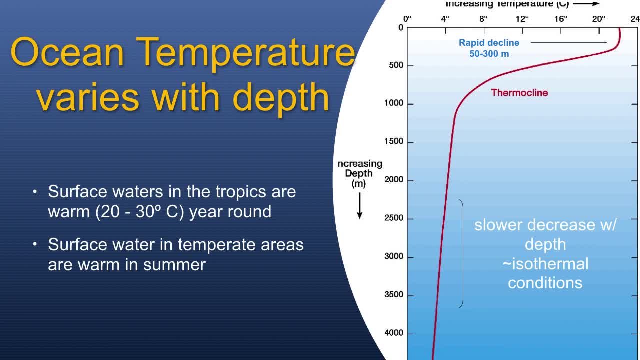 So we need to talk about how ocean temperature varies with depth. Surface waters in the tropics are warm year-round, at about 20 to 30 degrees C, And in the temperate regions of the ocean, surface waters are also warm during the summer. 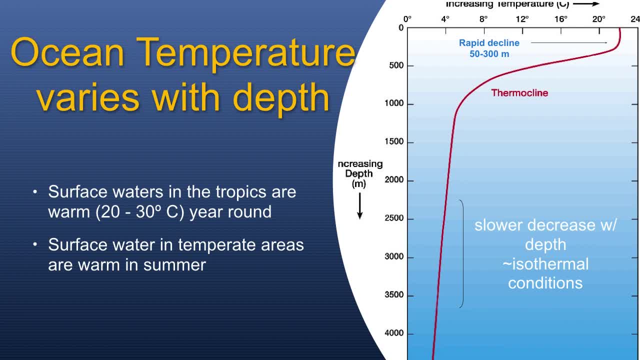 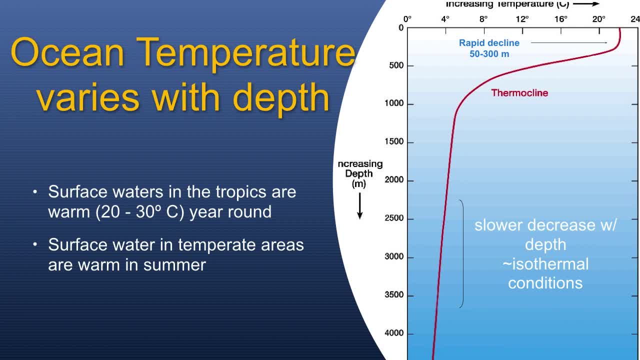 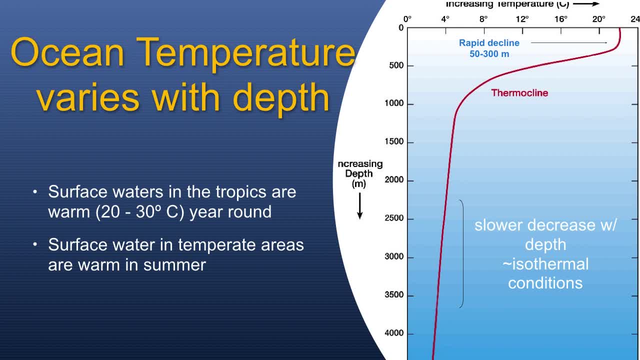 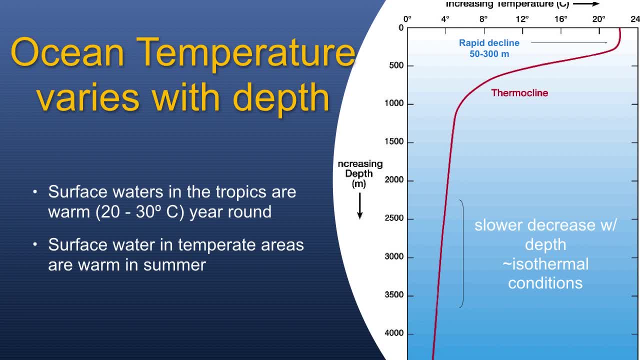 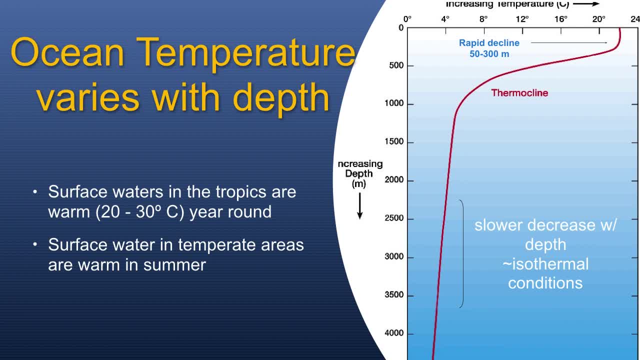 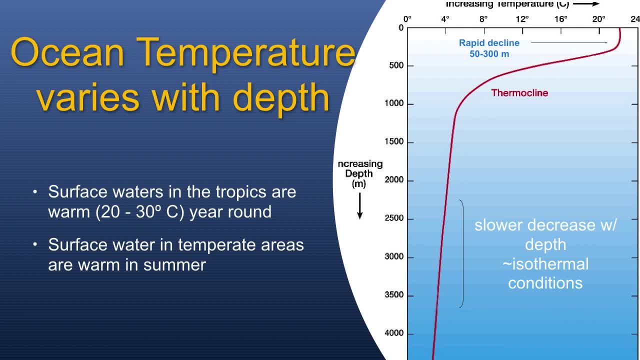 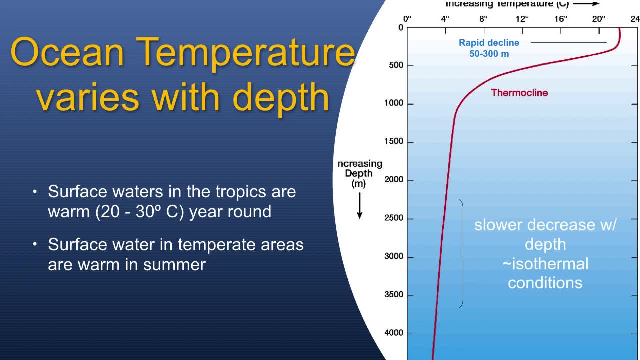 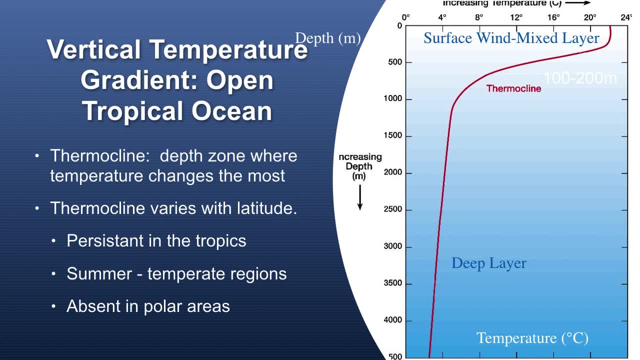 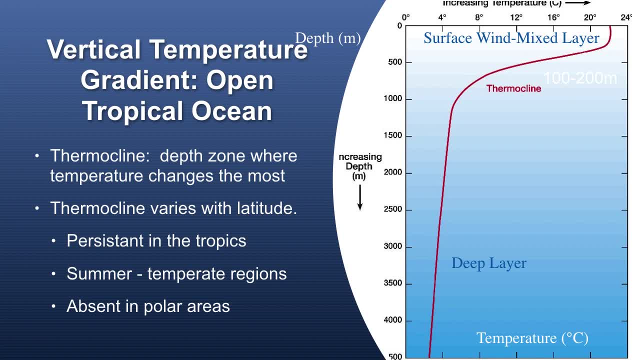 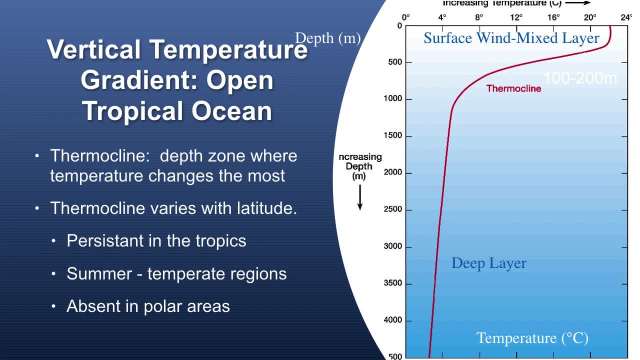 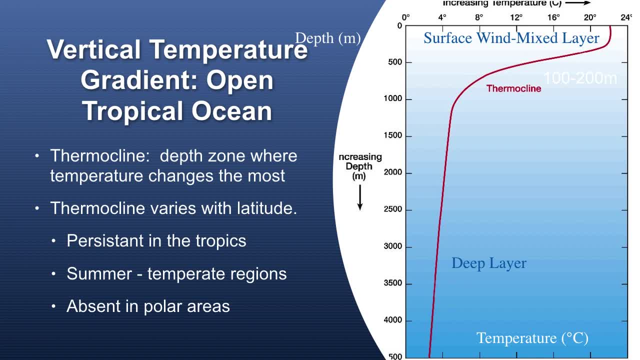 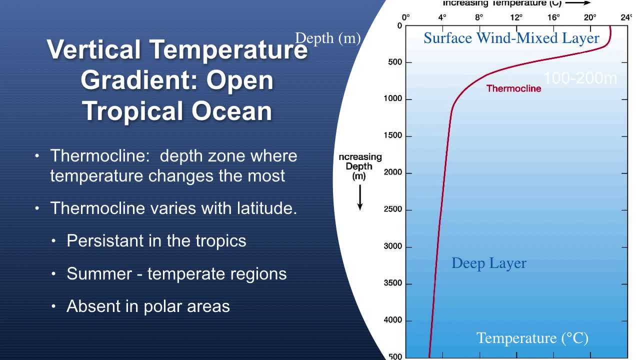 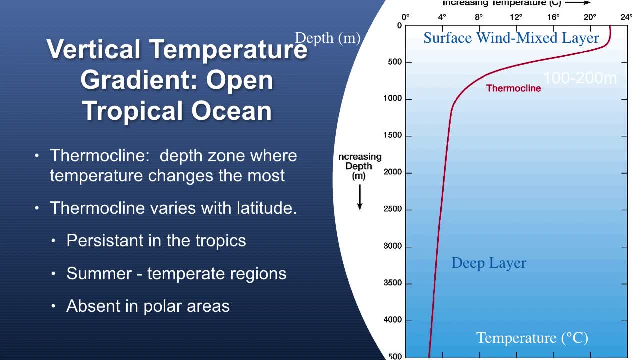 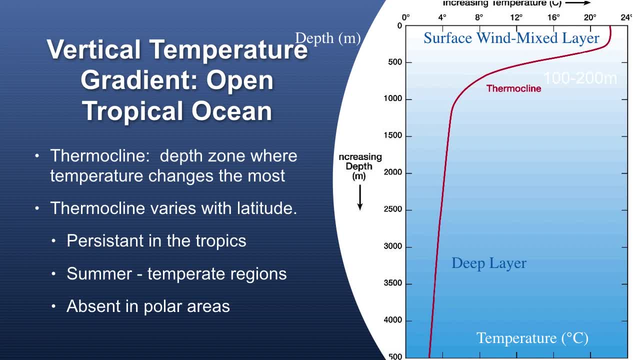 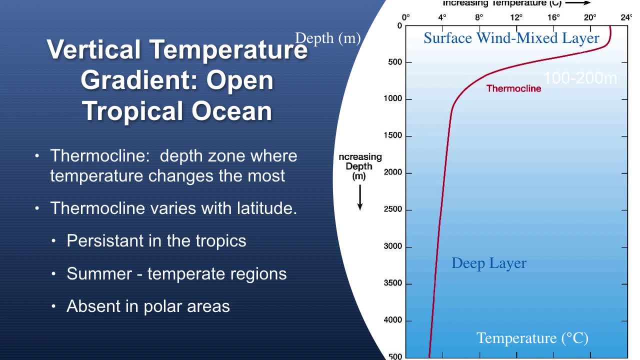 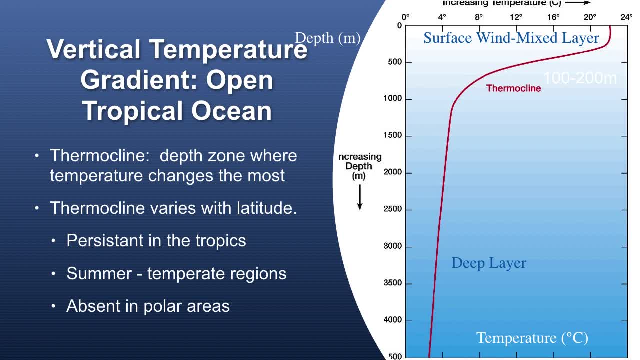 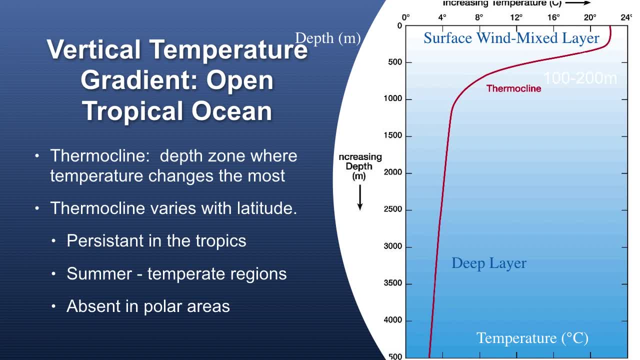 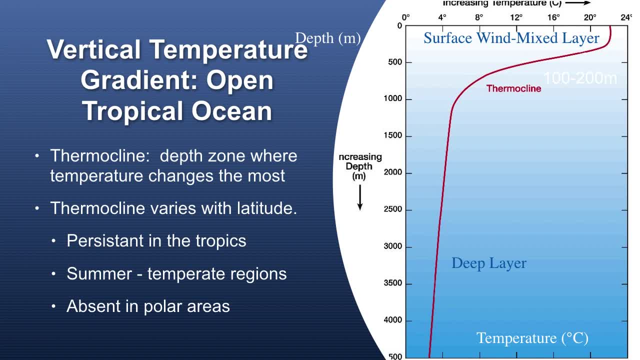 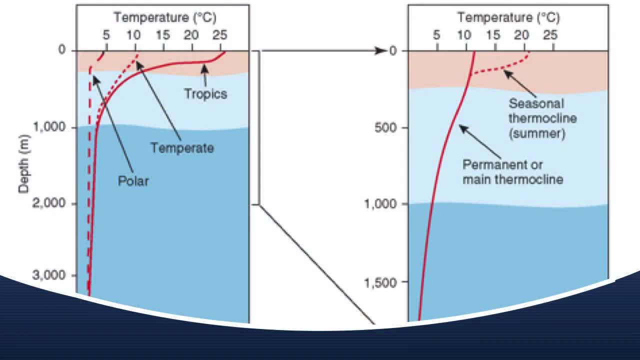 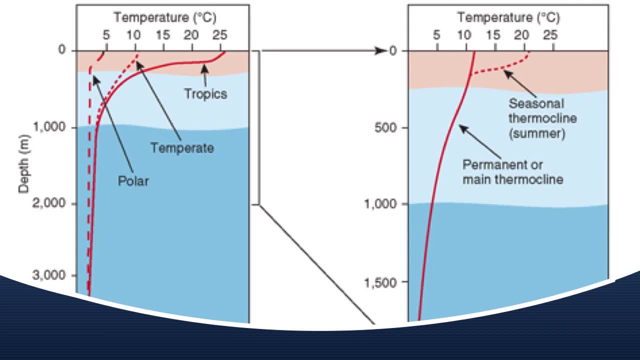 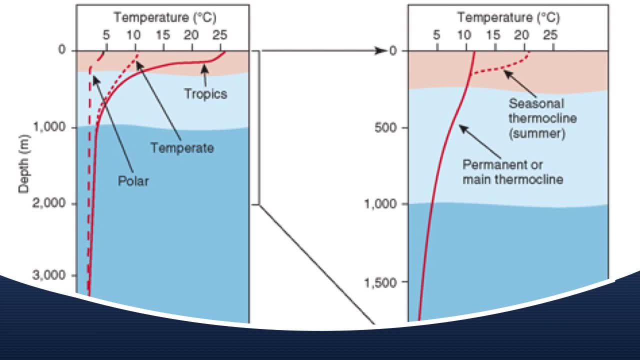 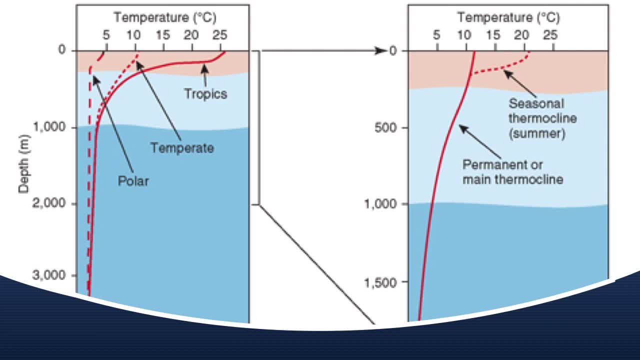 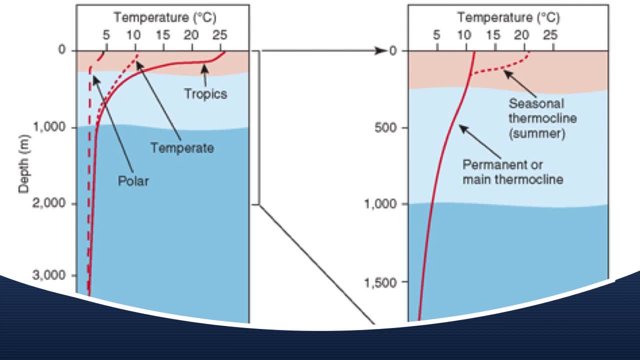 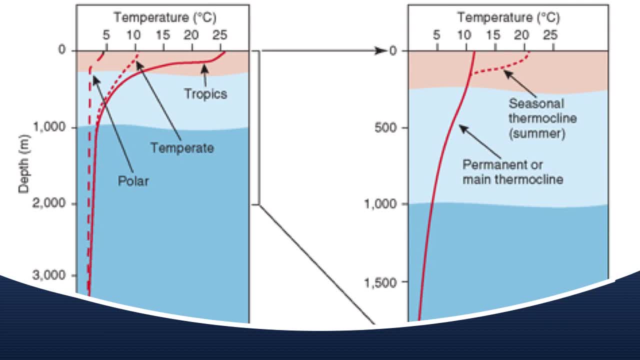 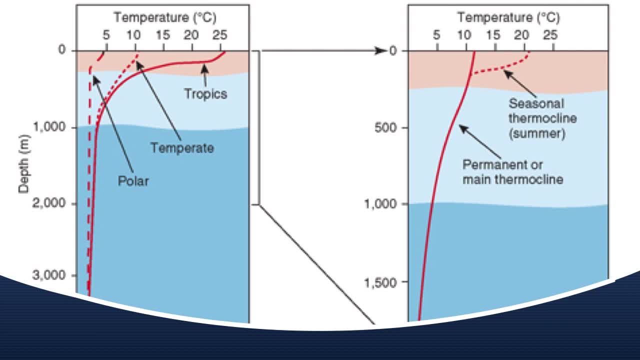 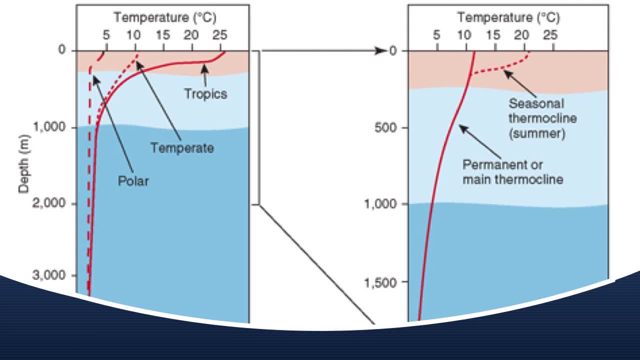 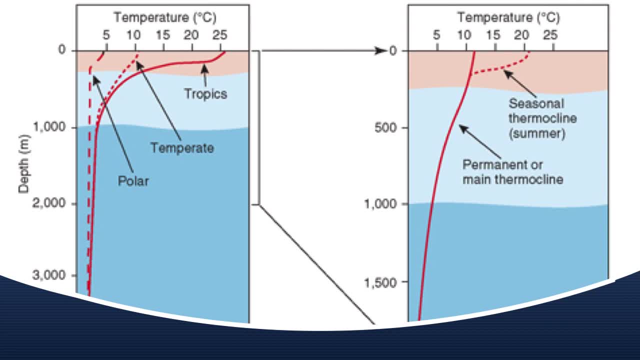 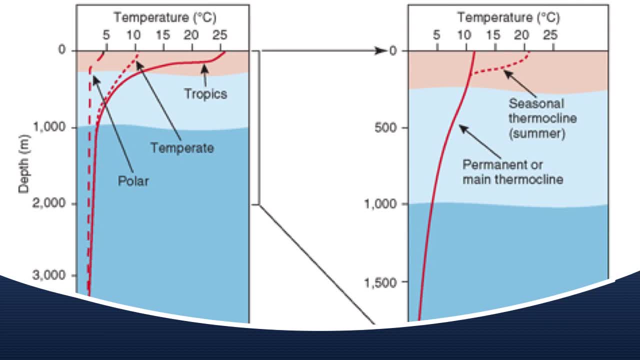 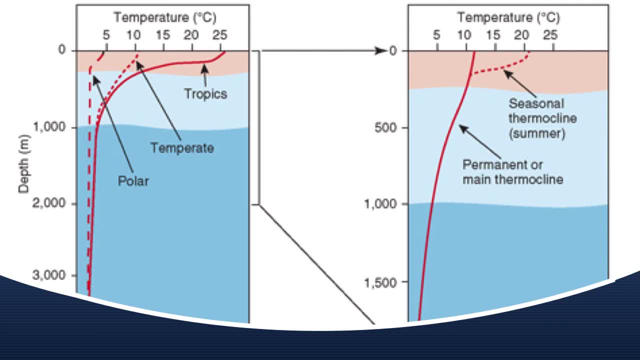 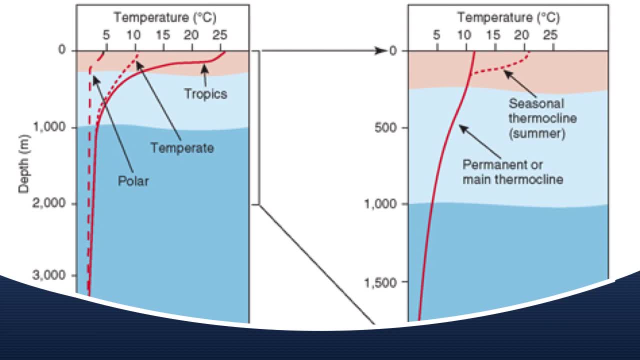 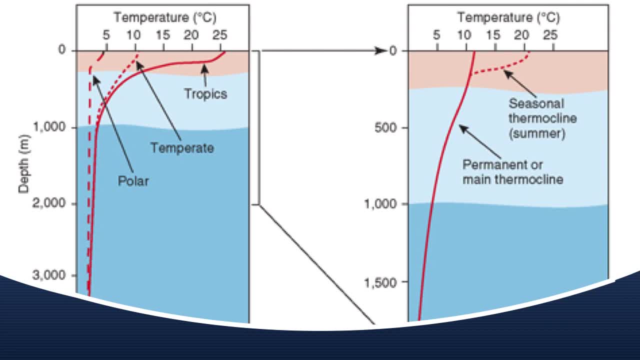 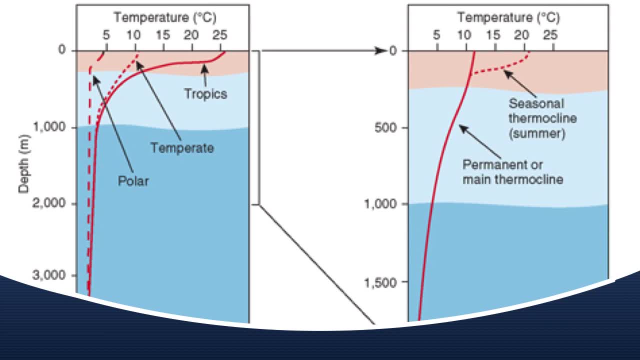 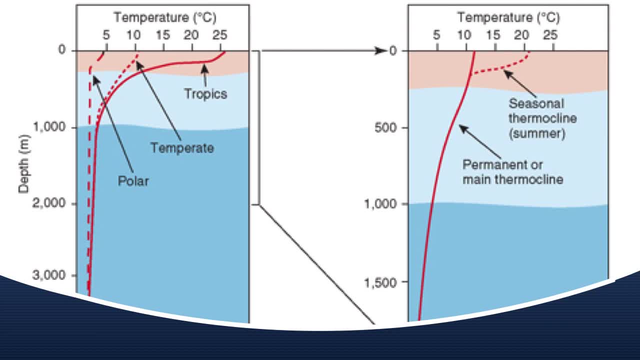 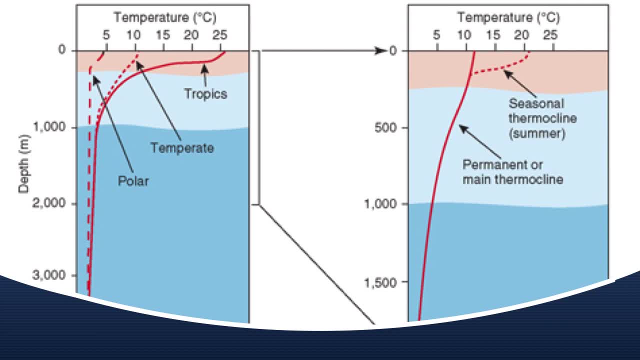 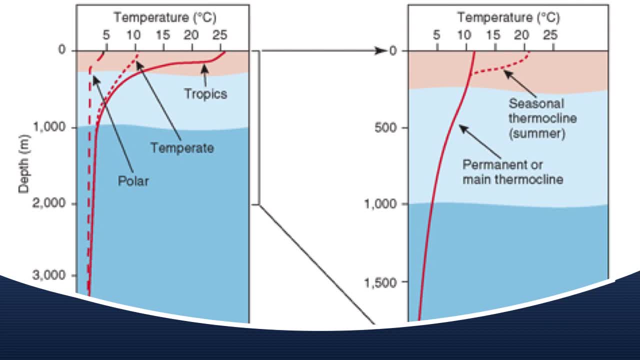 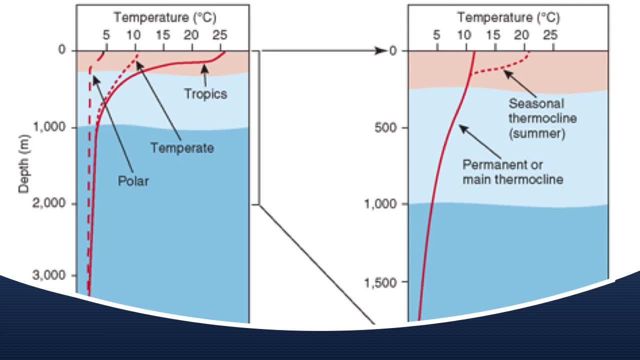 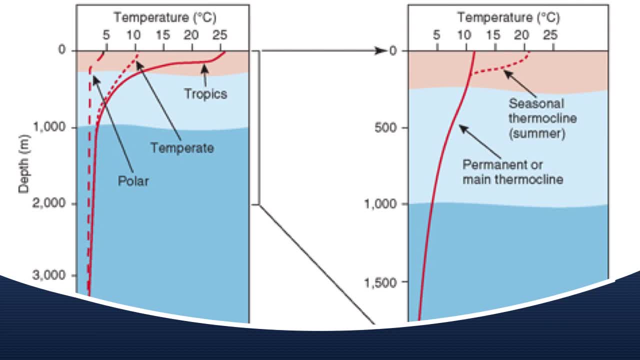 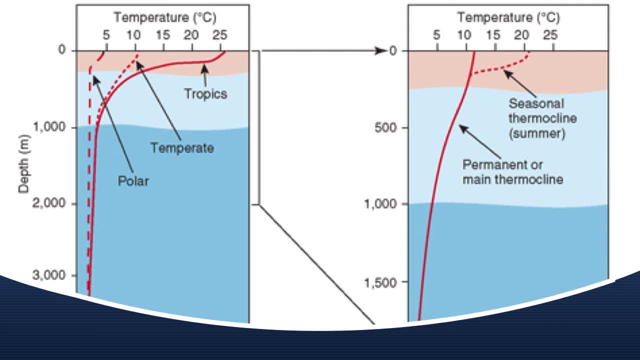 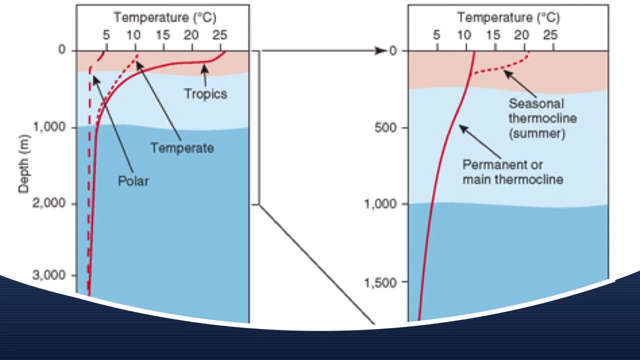 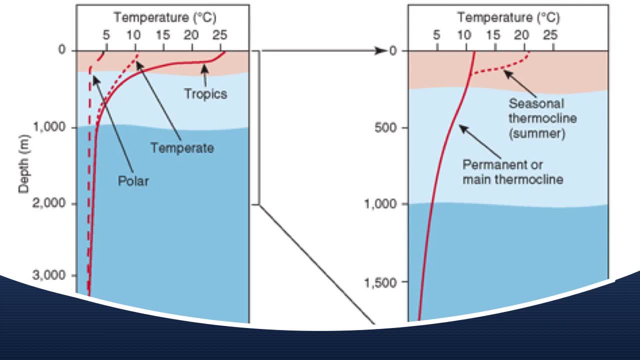 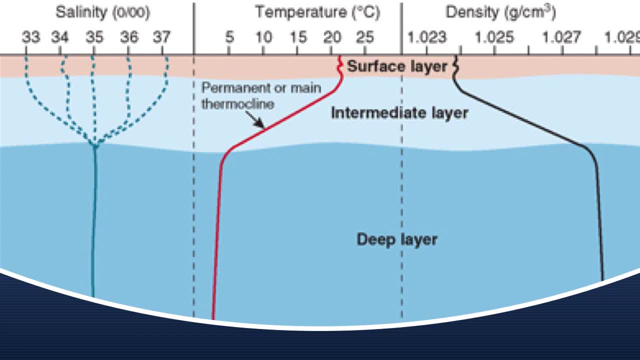 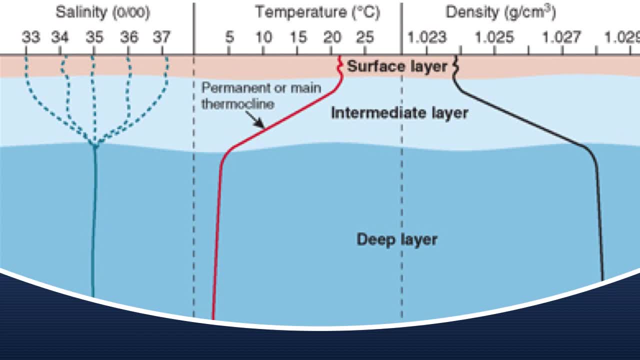 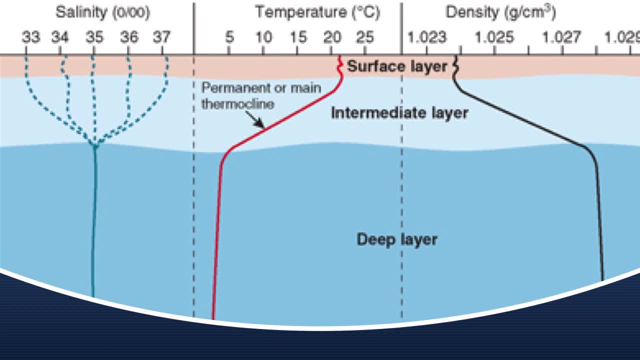 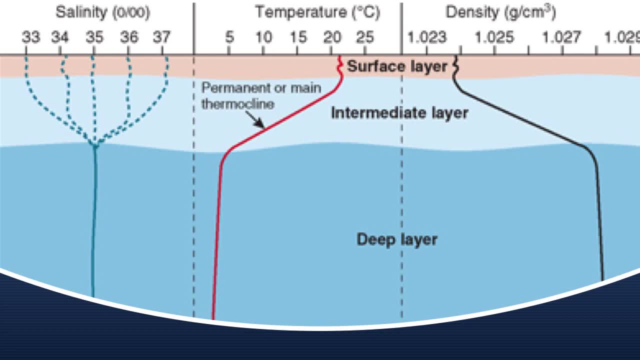 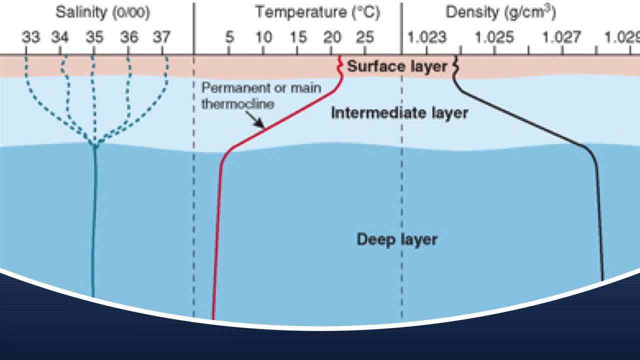 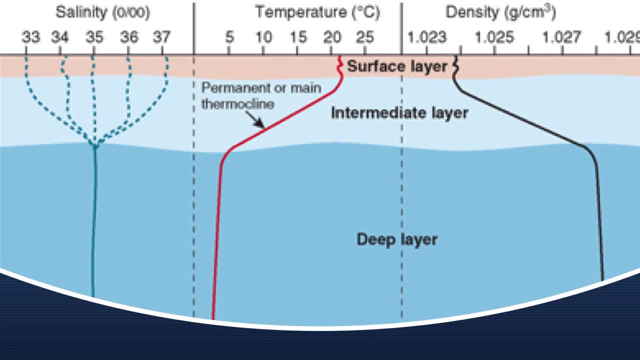 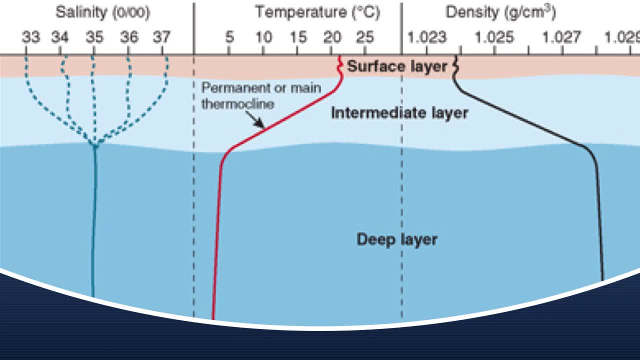 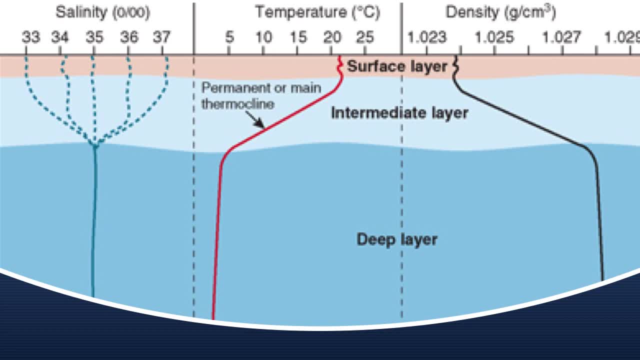 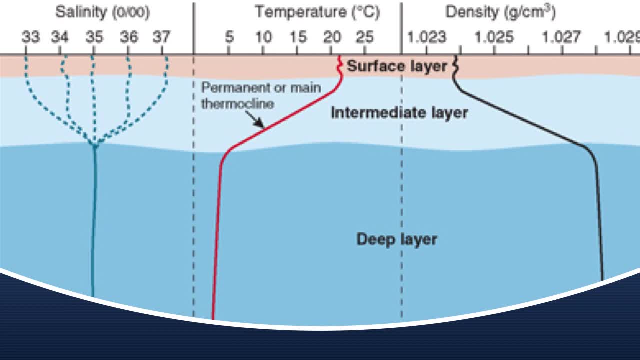 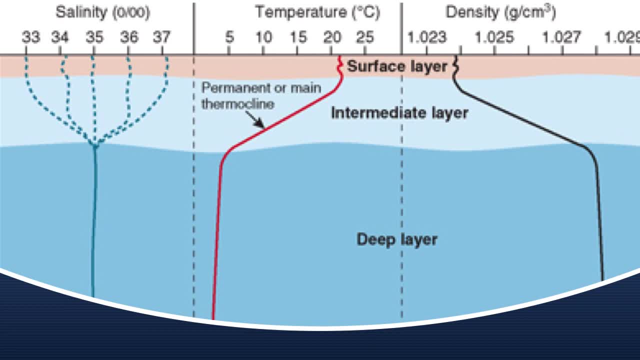 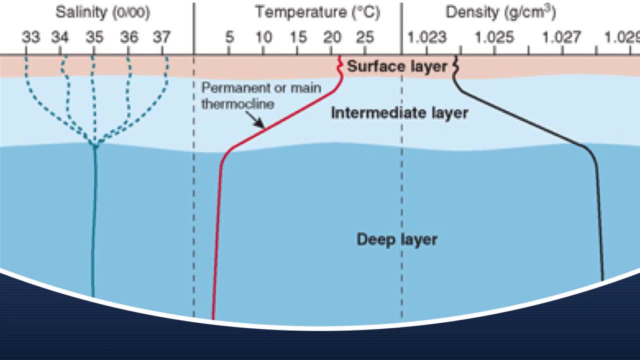 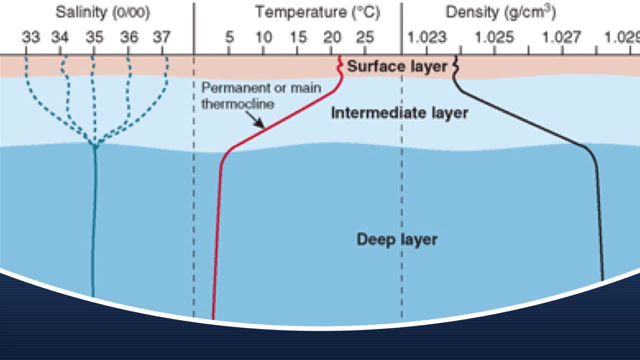 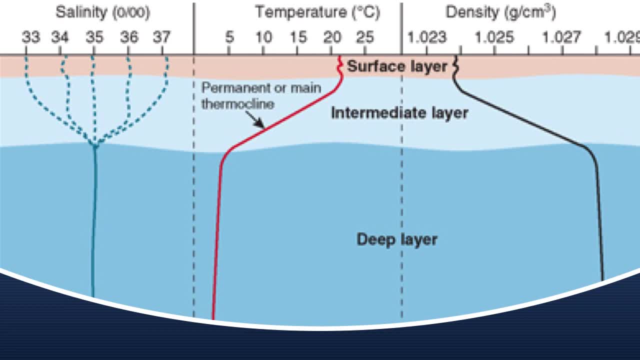 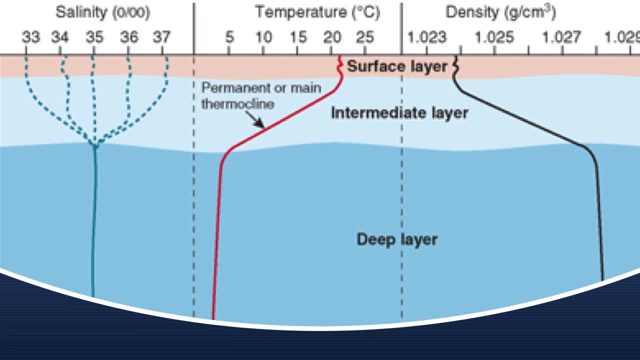 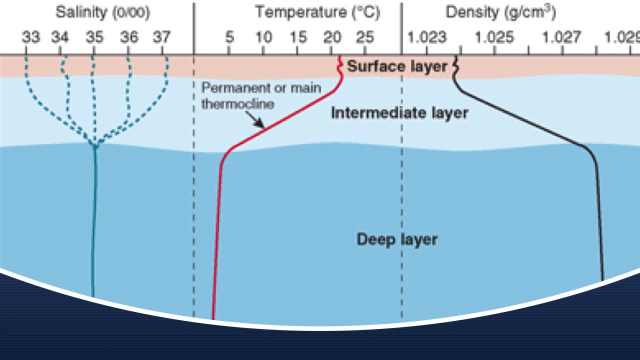 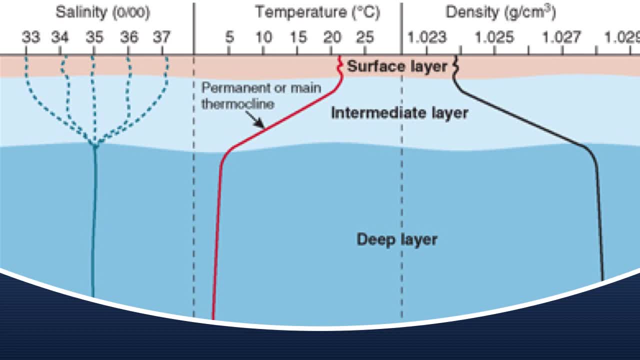 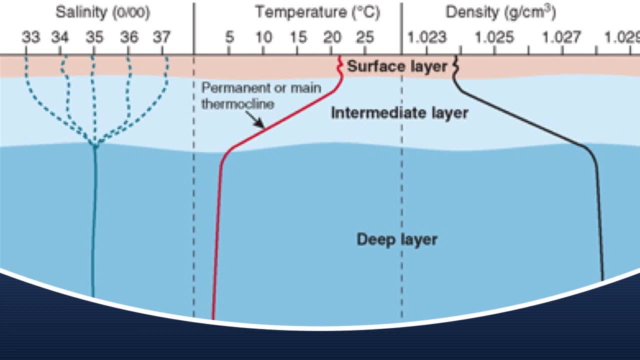 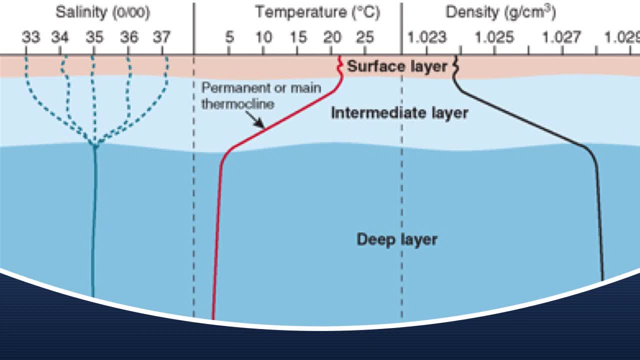 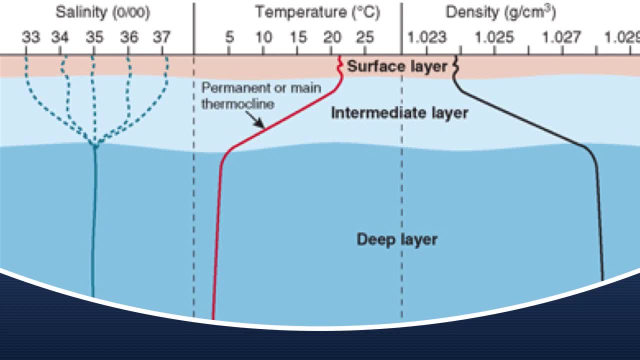 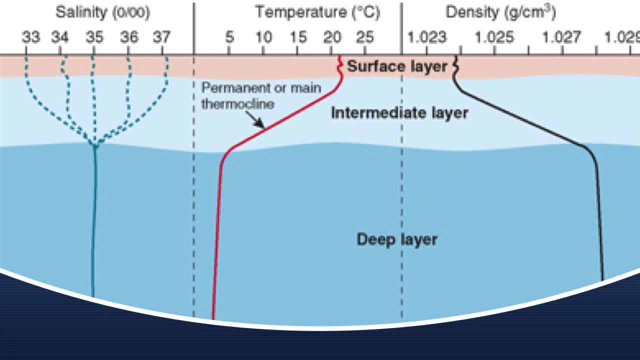 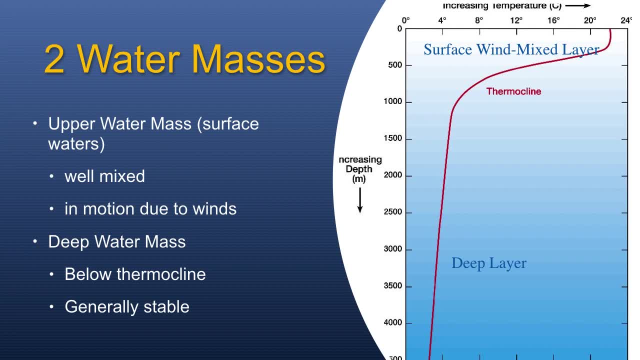 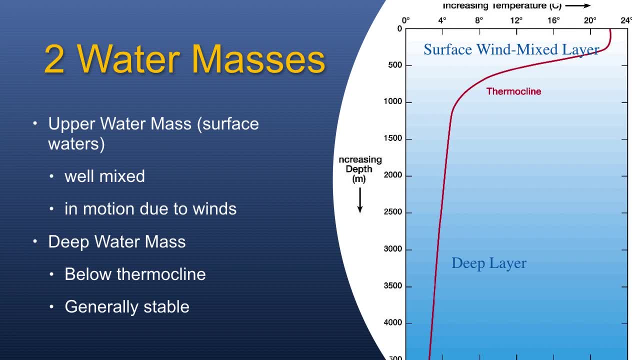 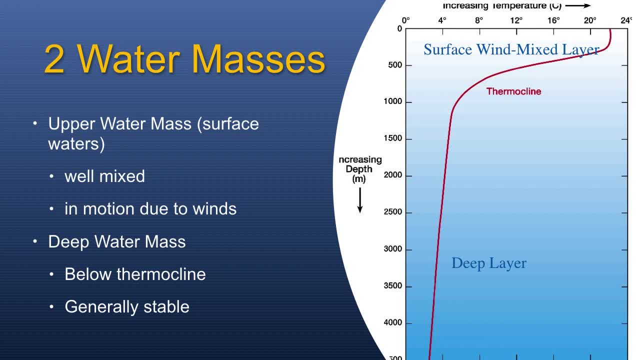 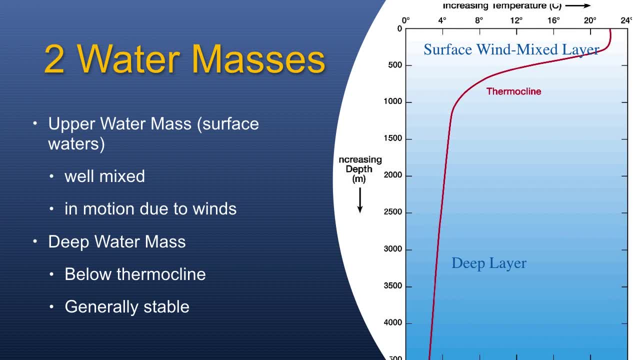 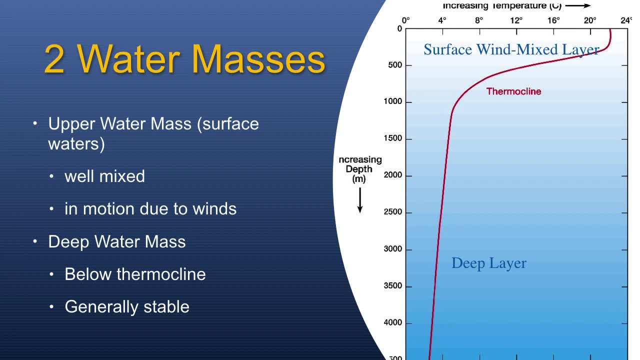 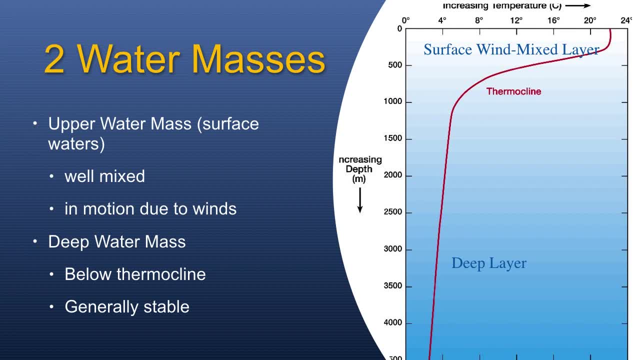 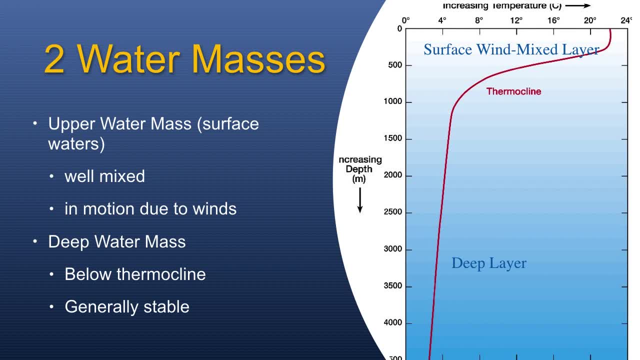 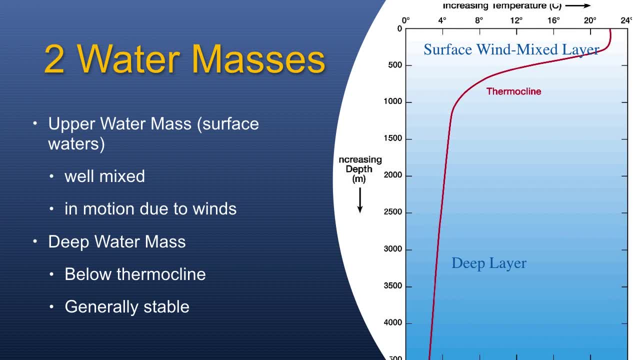 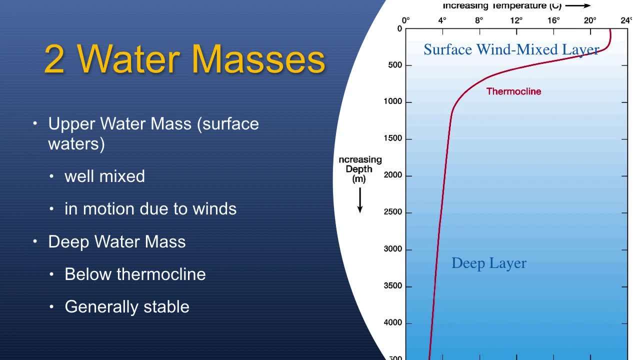 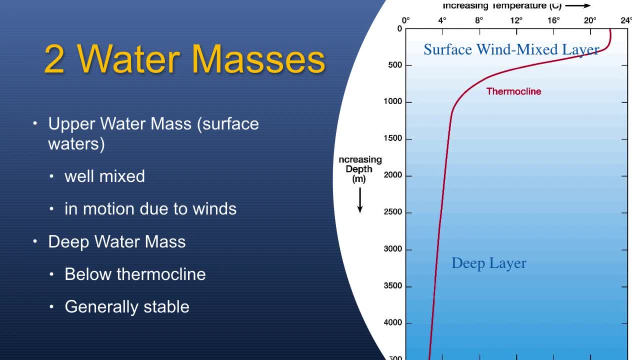 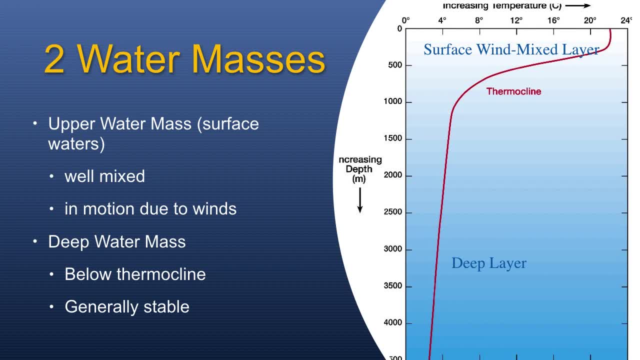 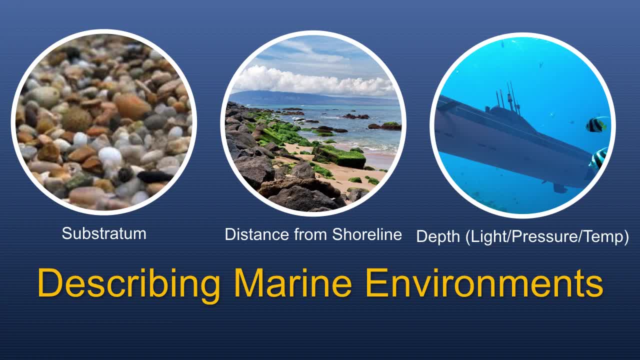 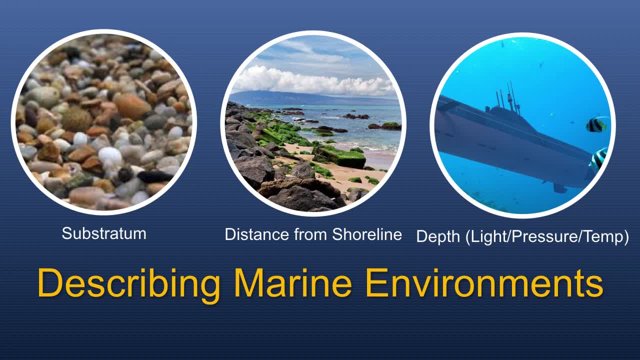 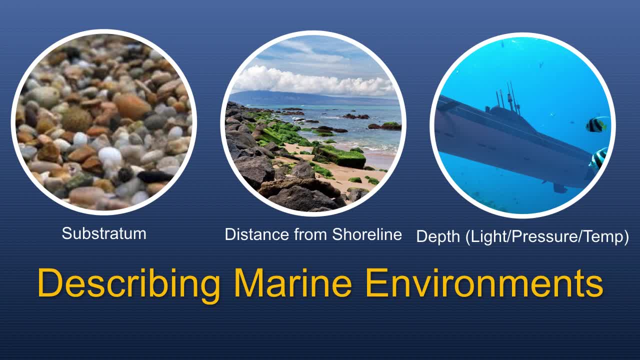 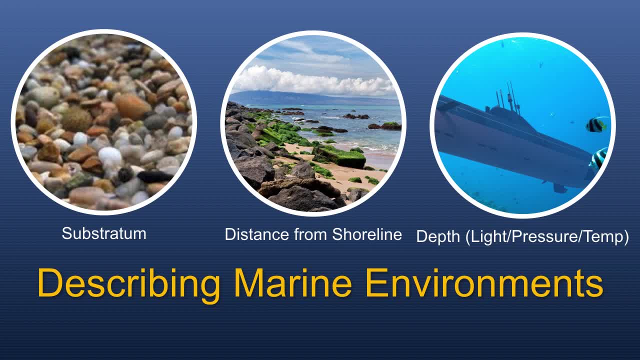 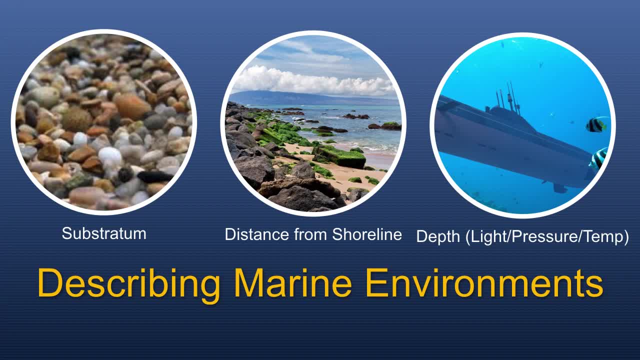 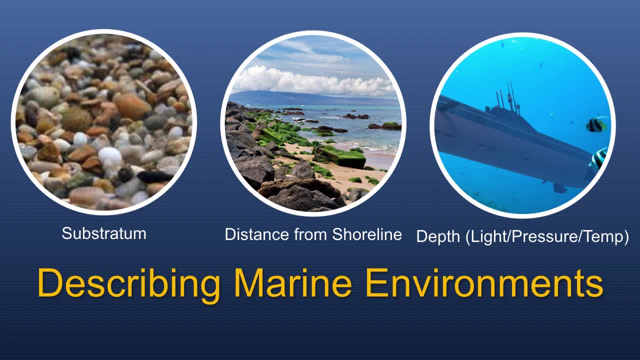 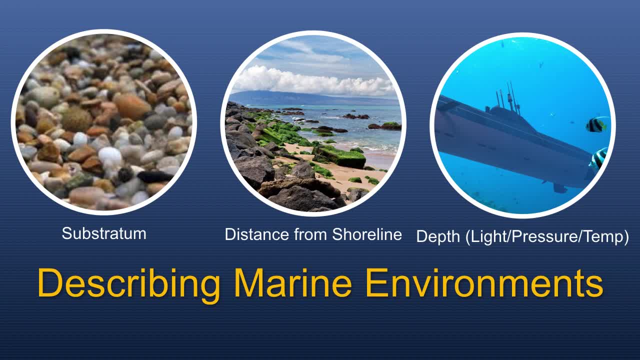 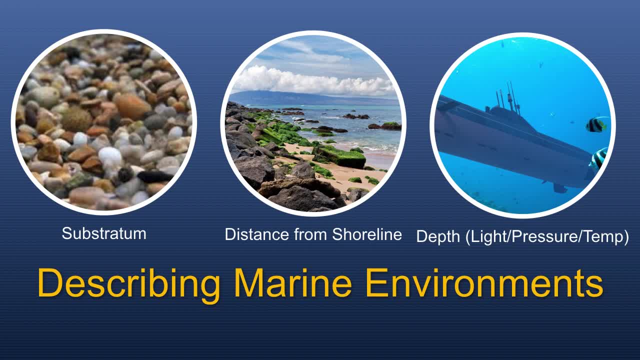 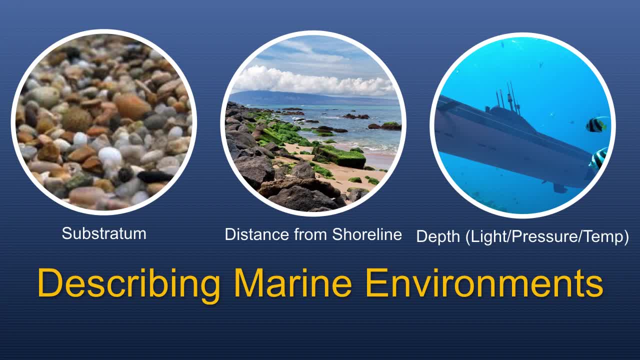 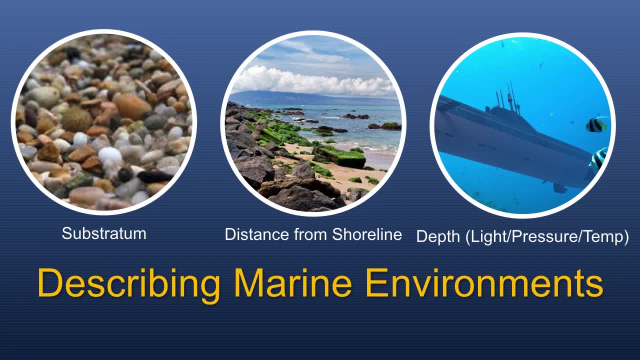 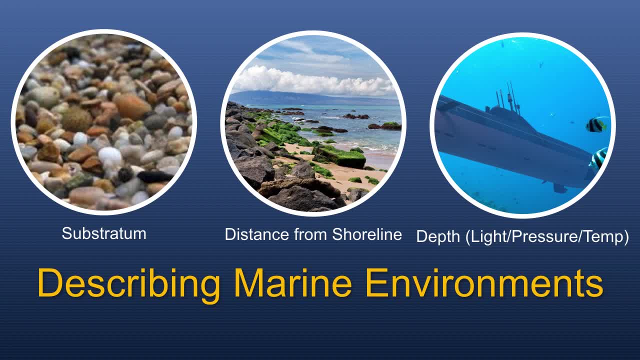 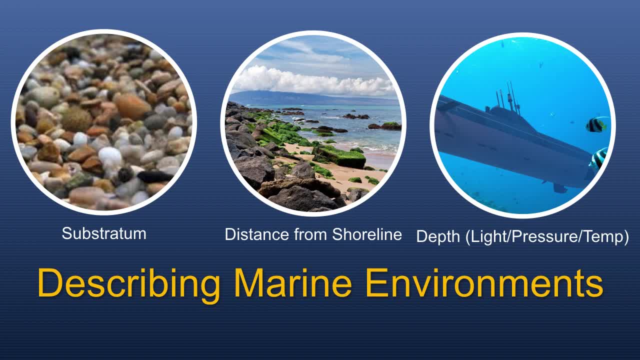 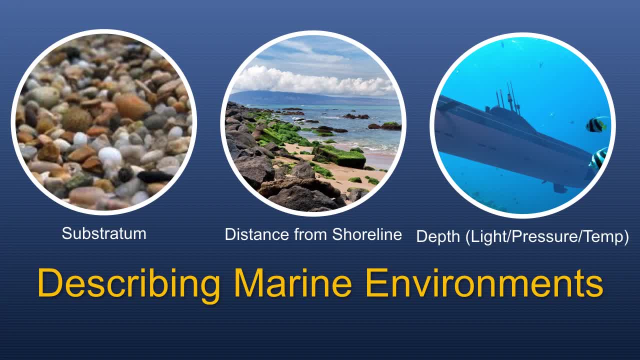 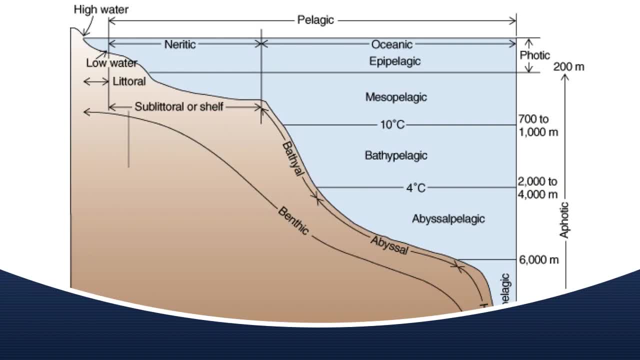 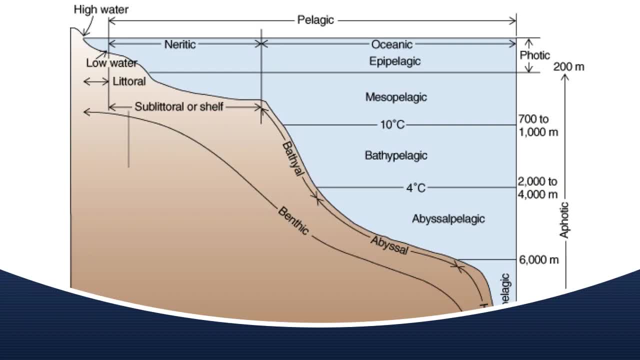 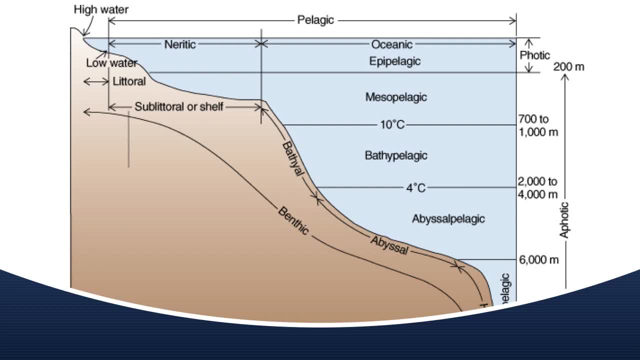 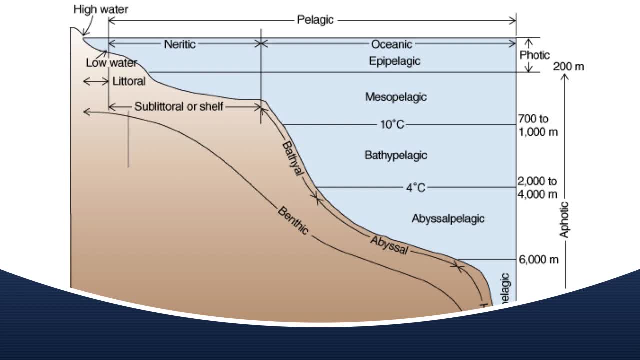 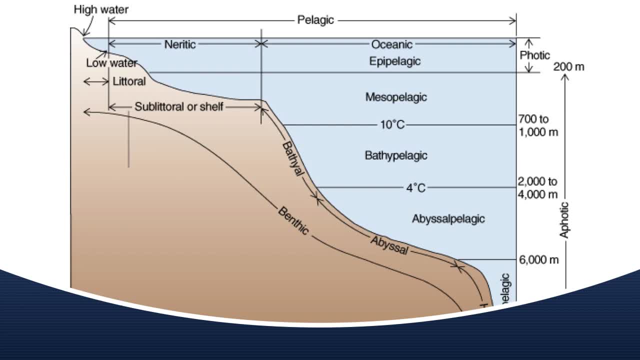 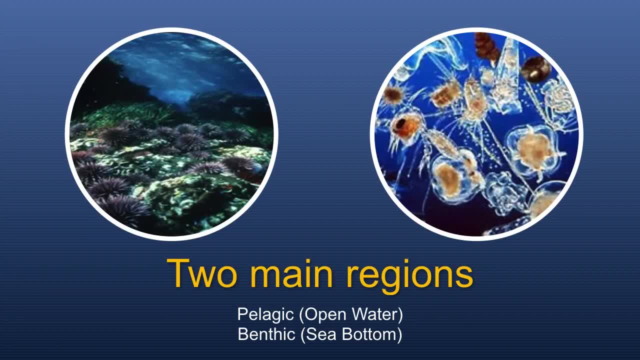 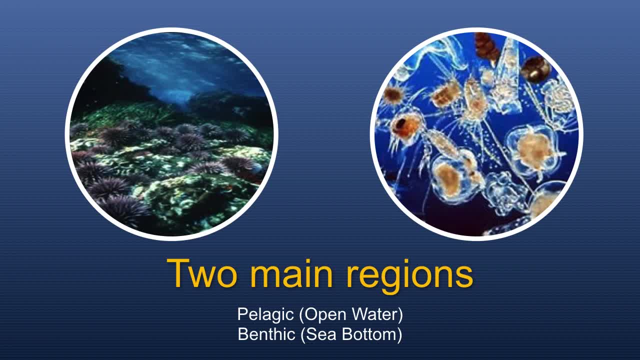 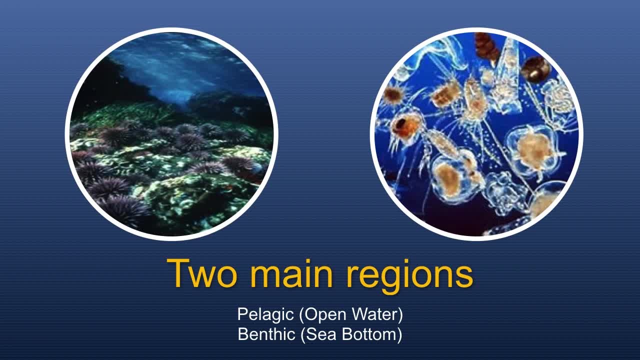 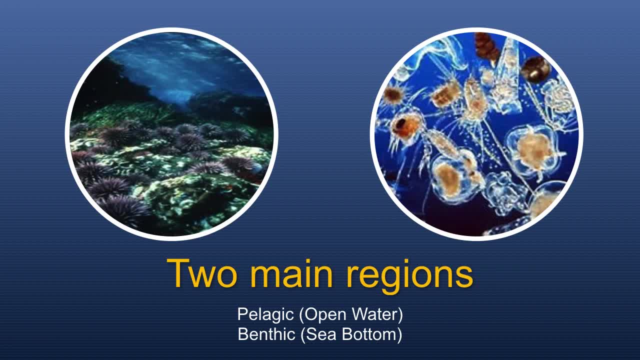 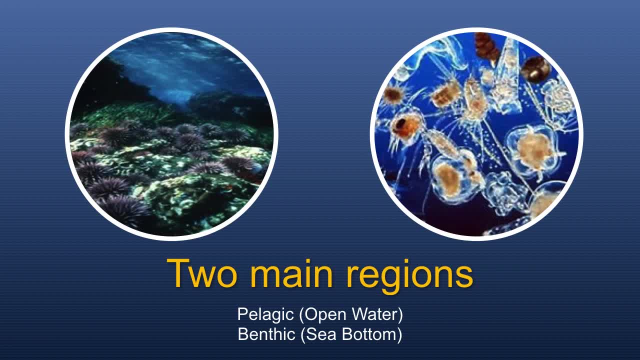 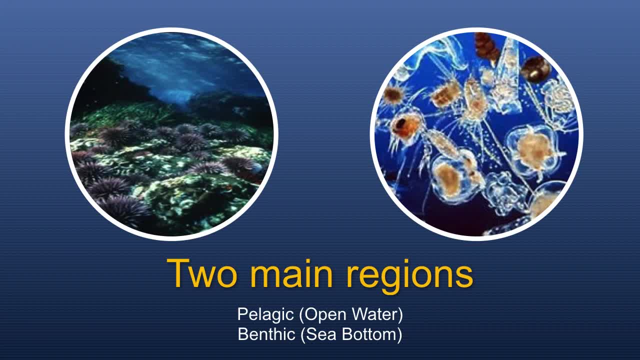 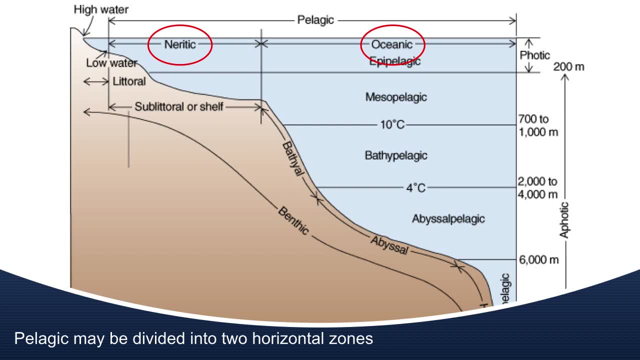 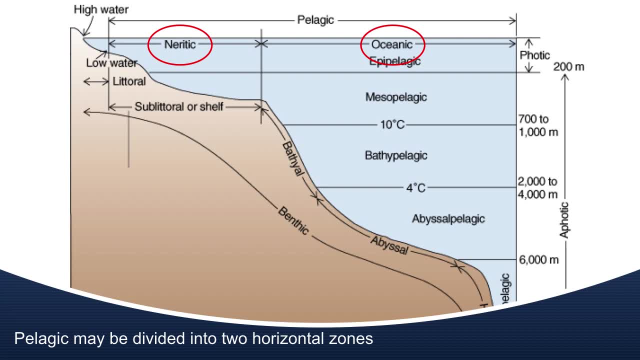 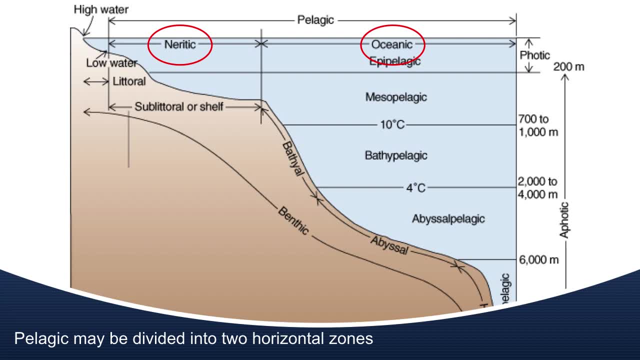 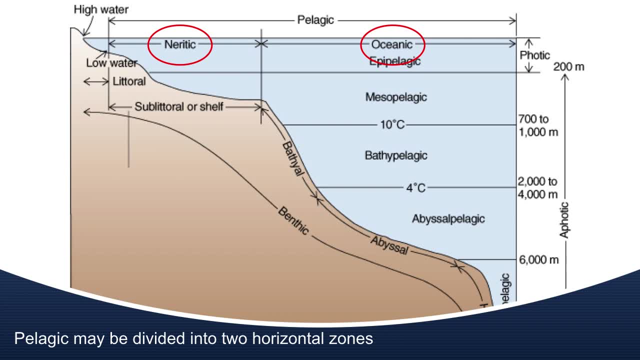 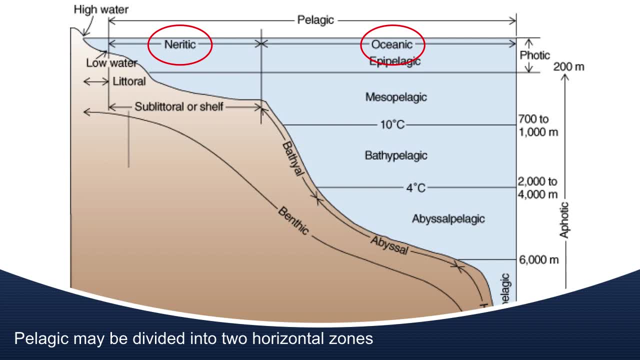 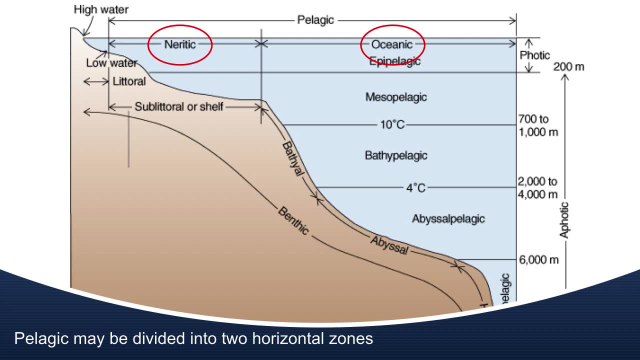 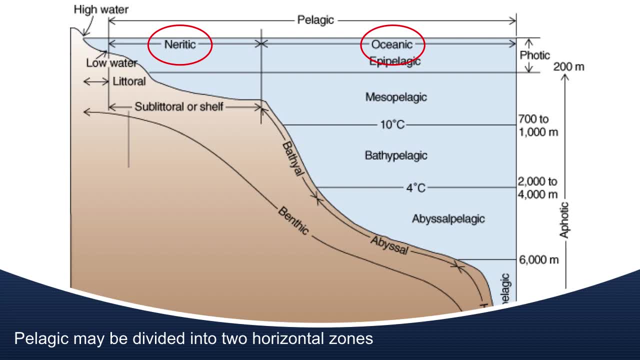 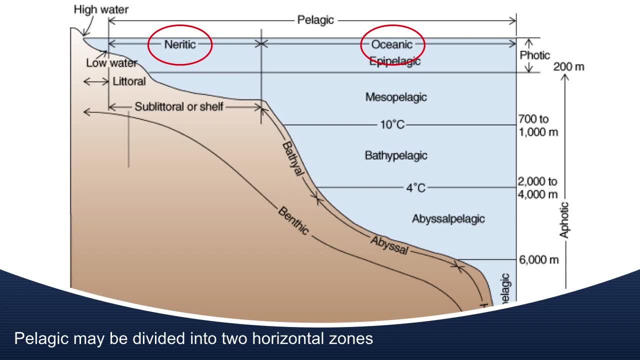 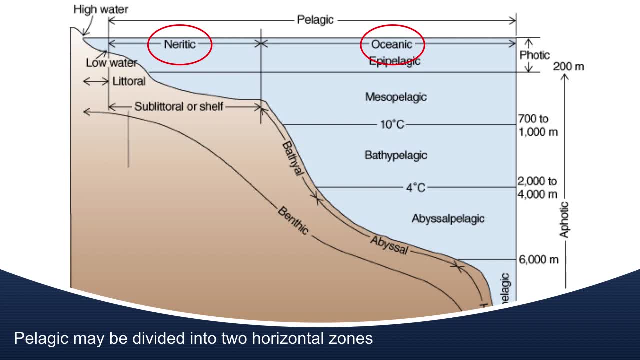 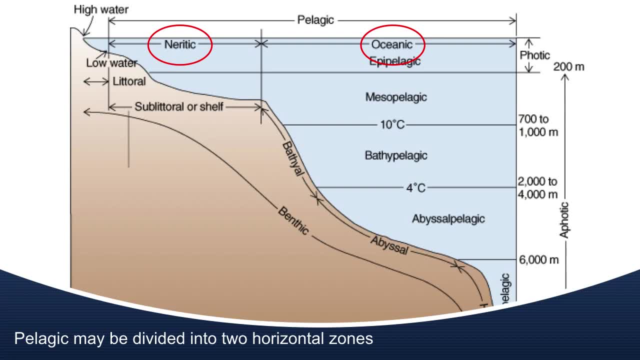 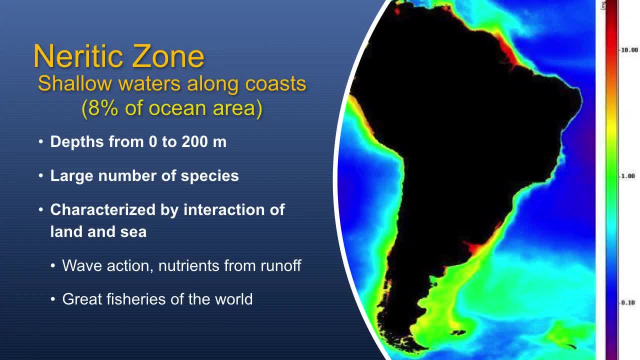 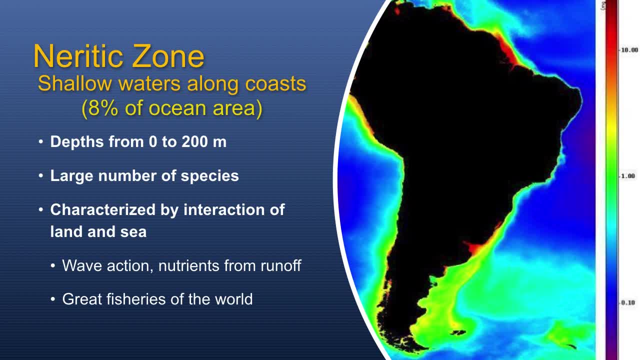 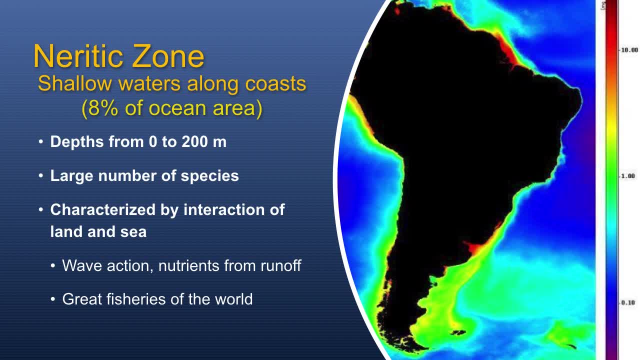 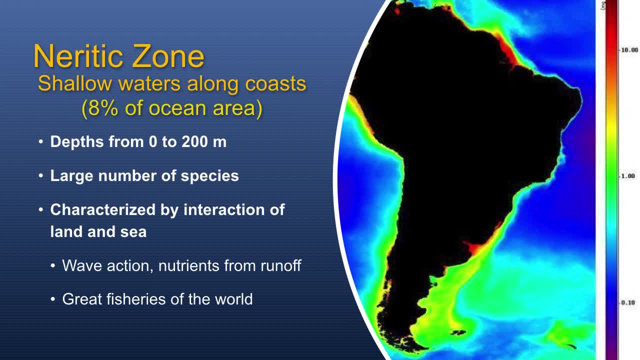 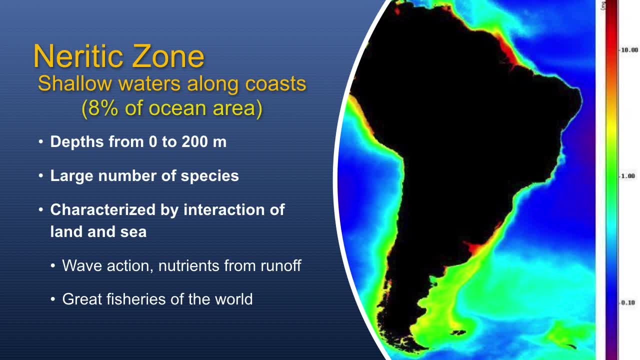 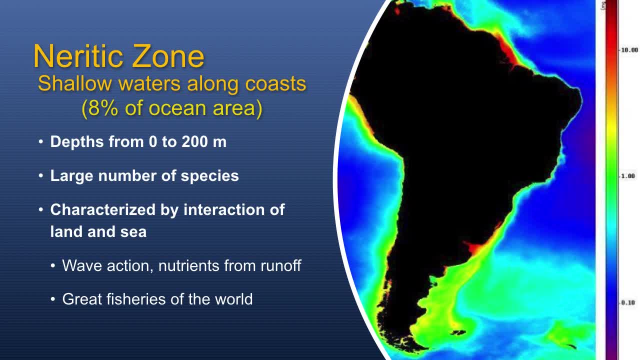 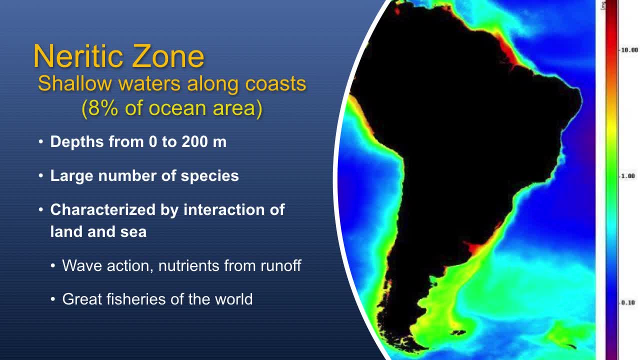 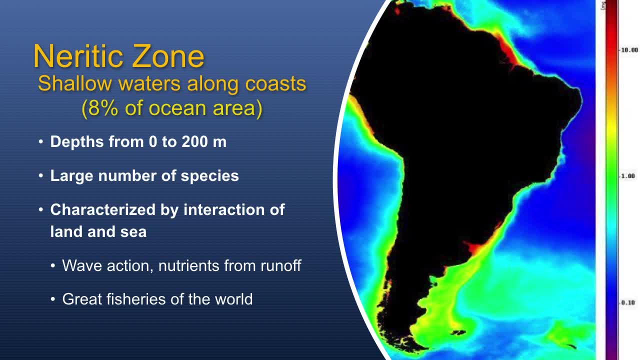 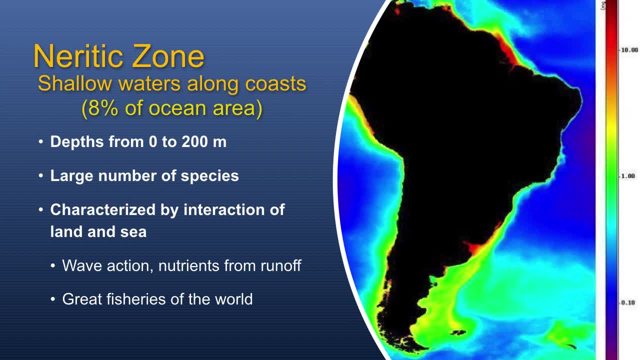 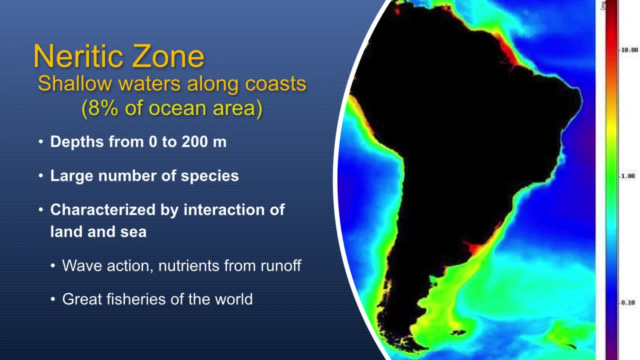 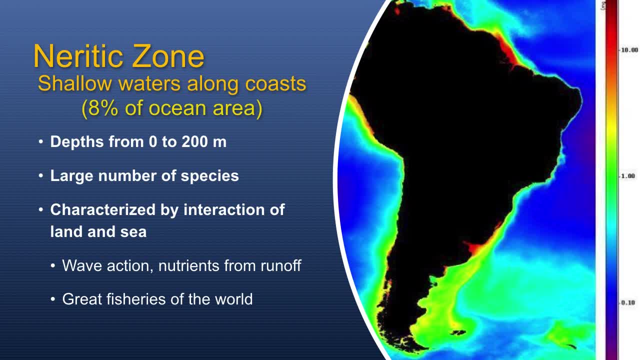 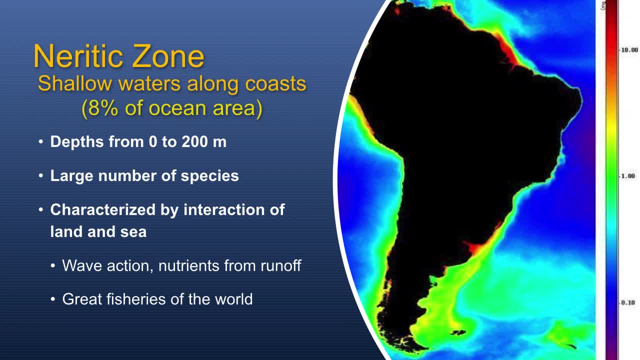 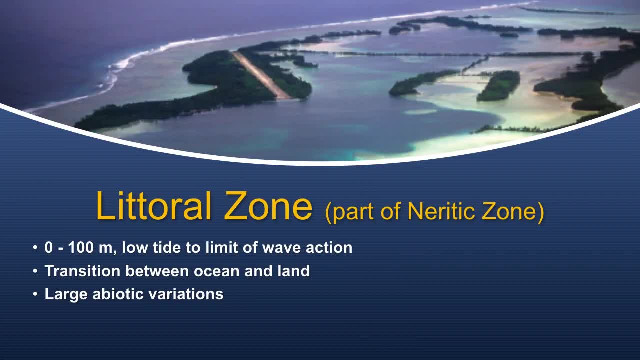 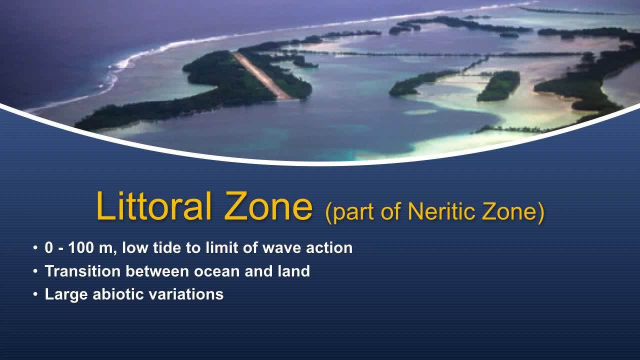 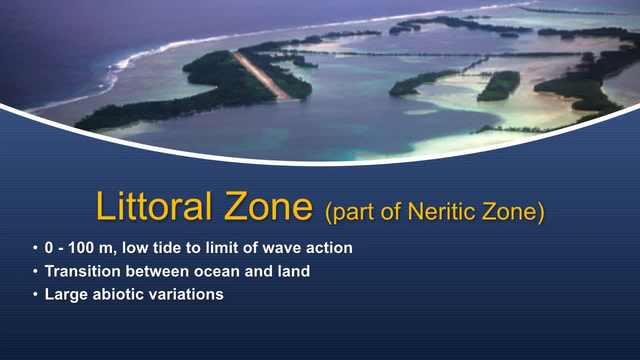 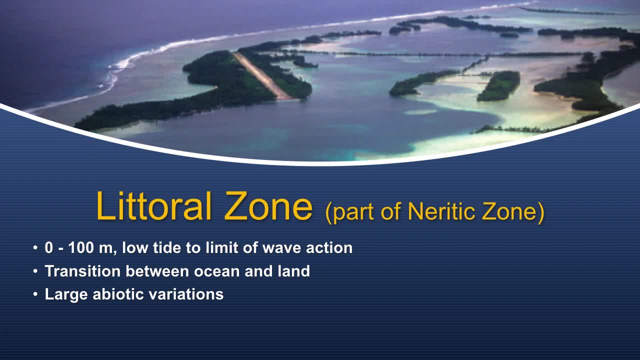 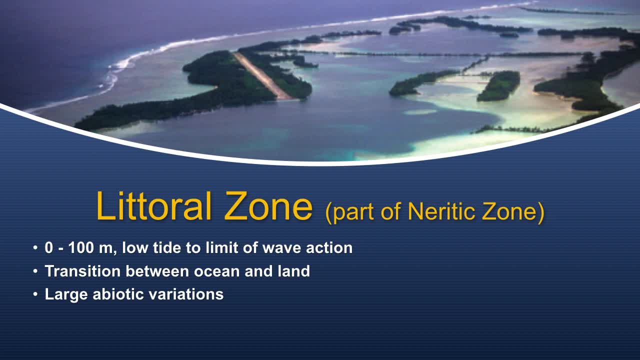 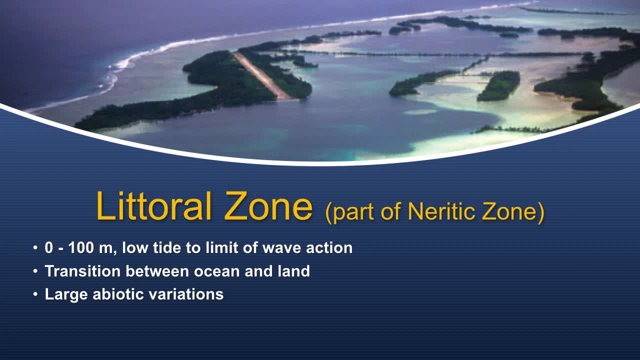 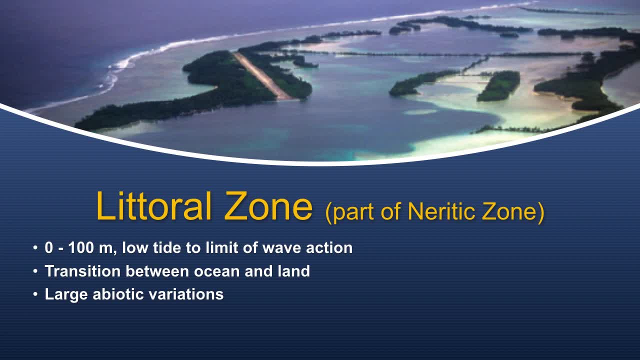 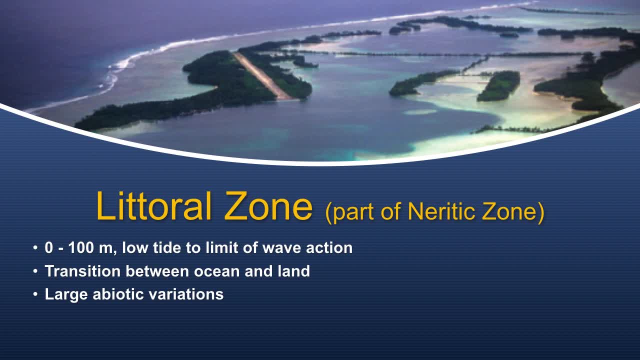 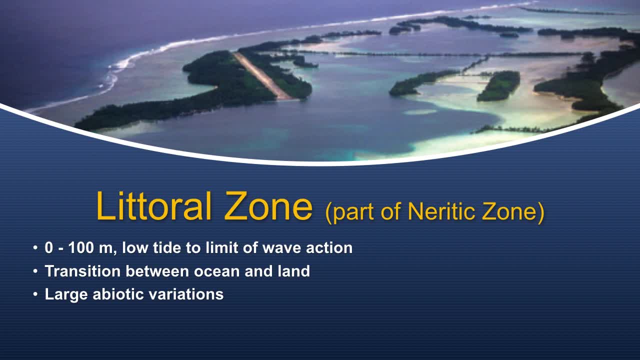 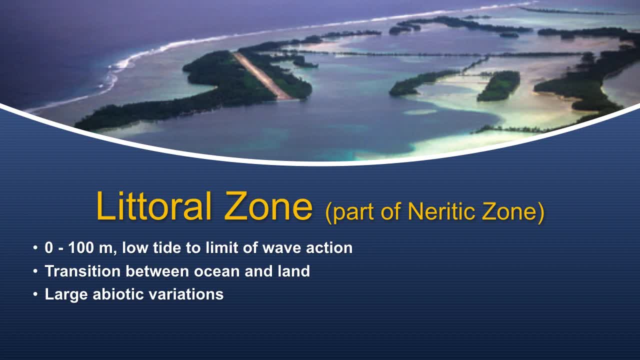 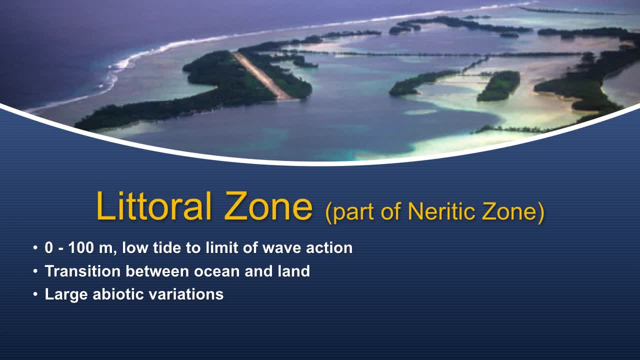 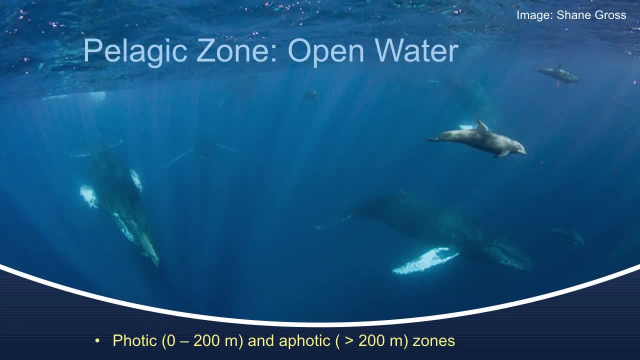 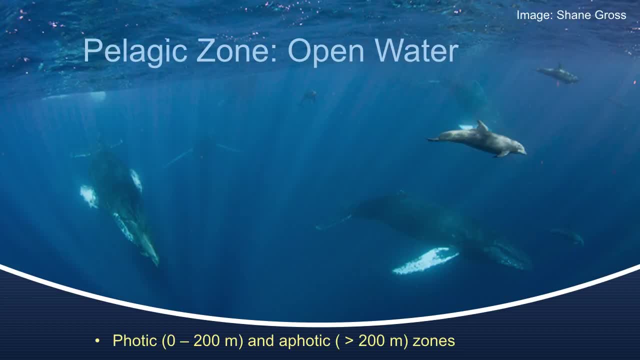 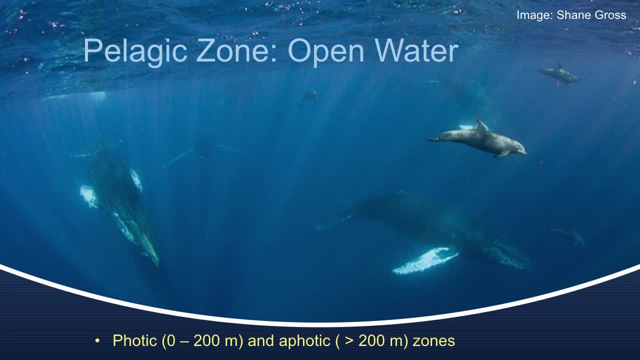 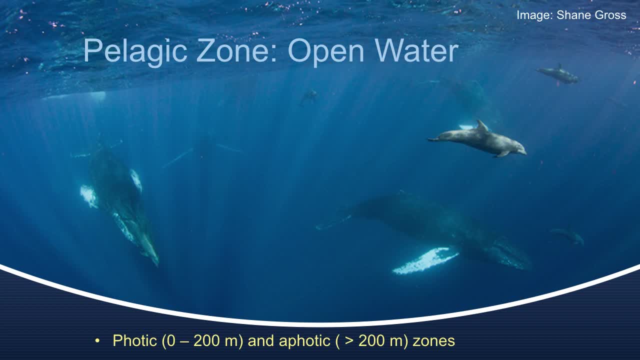 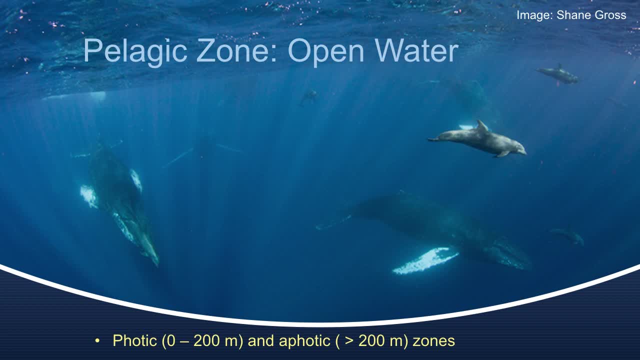 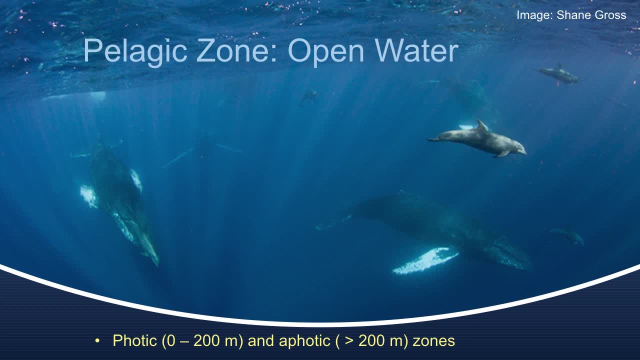 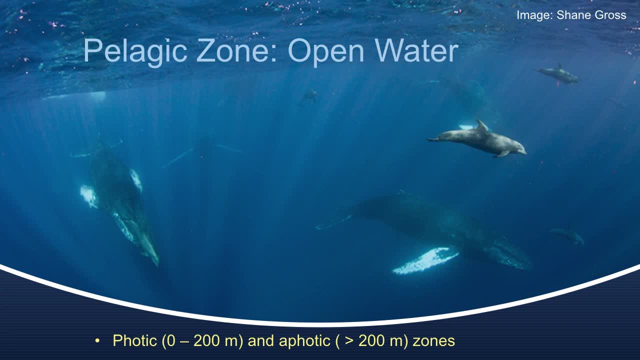 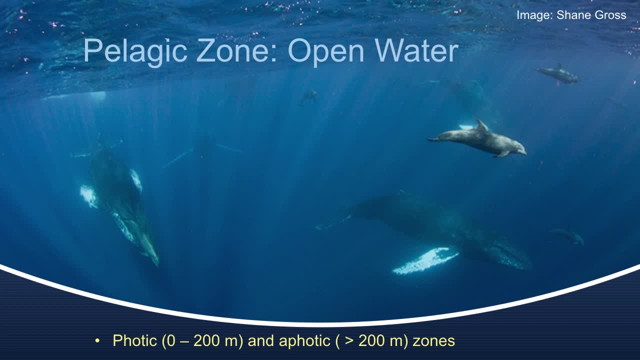 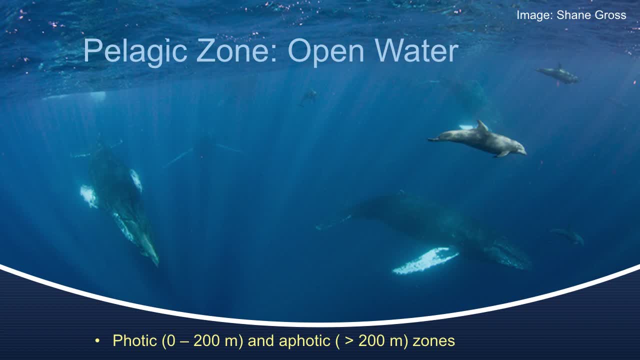 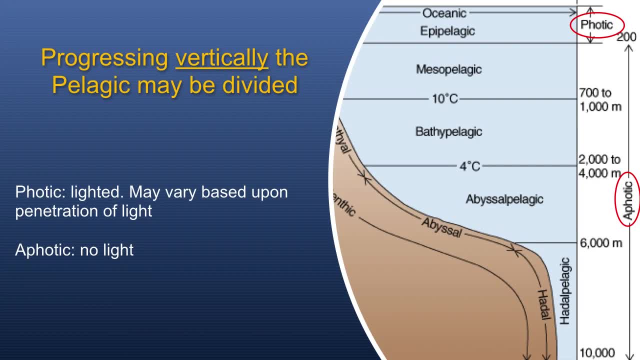 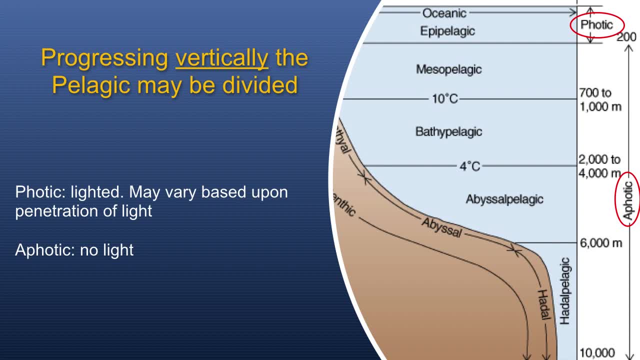 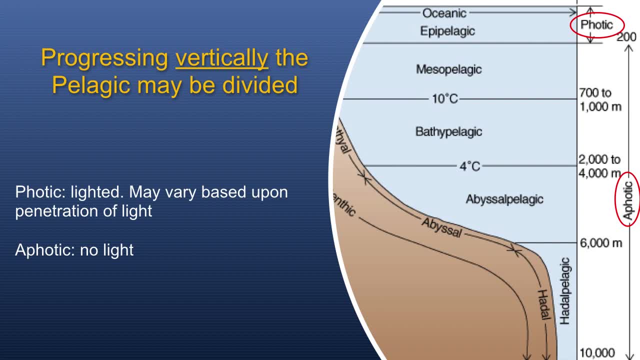 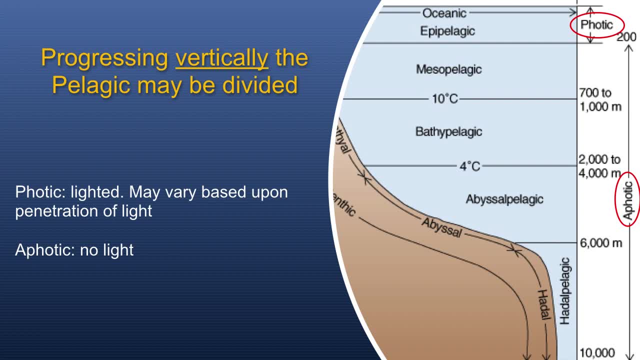 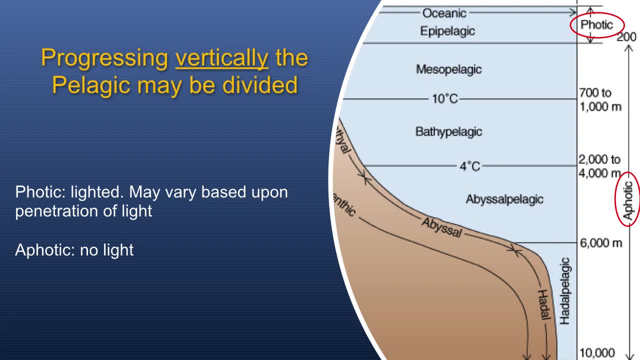 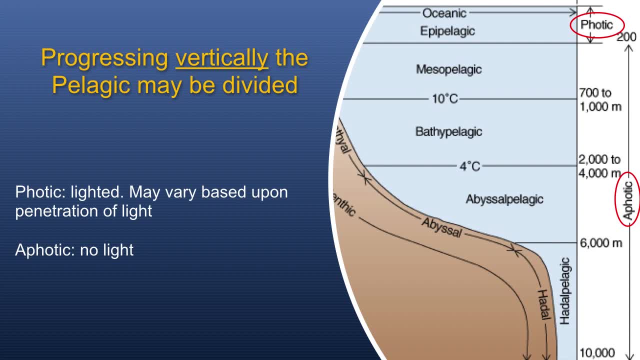 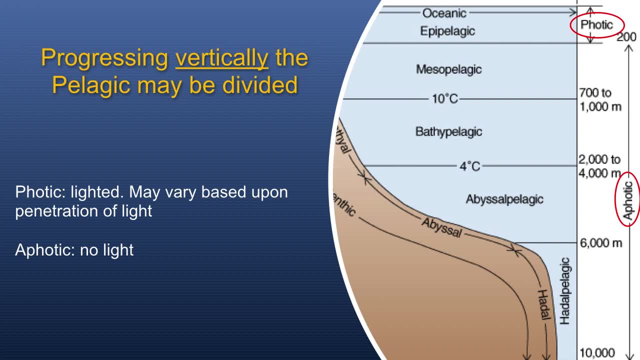 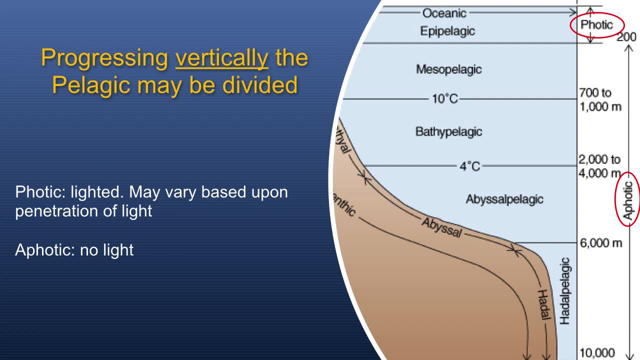 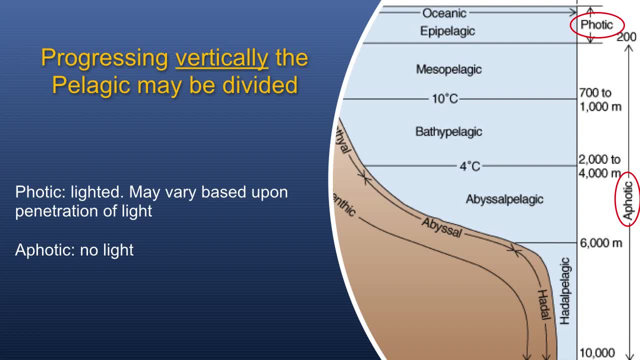 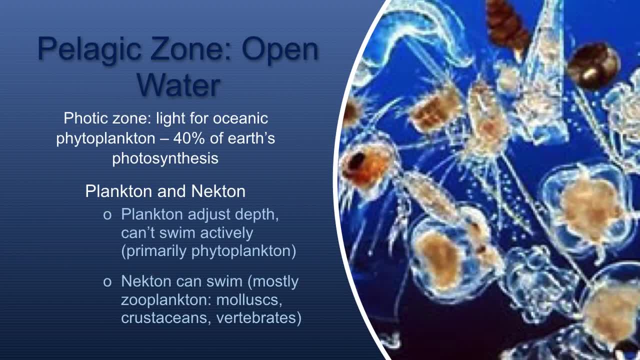 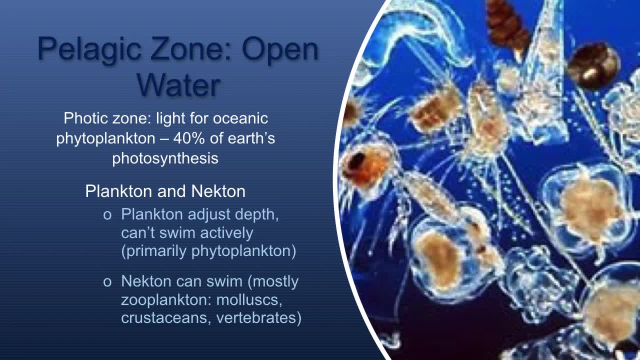 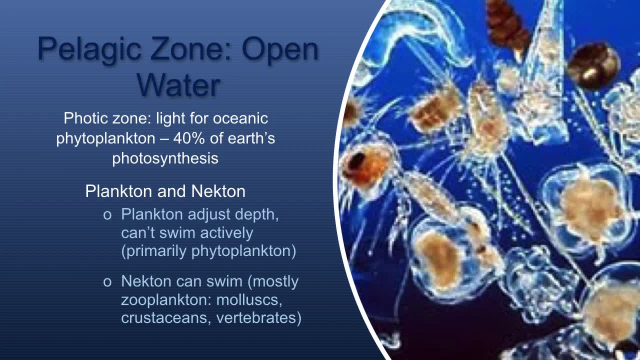 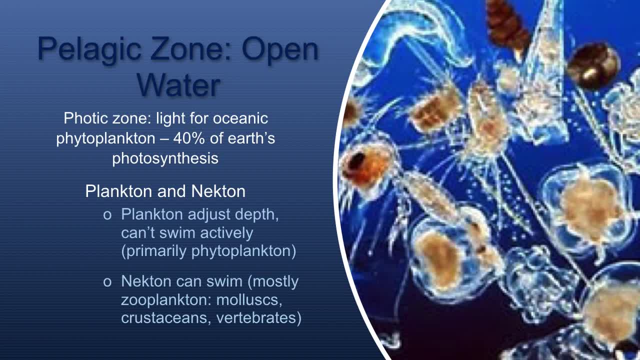 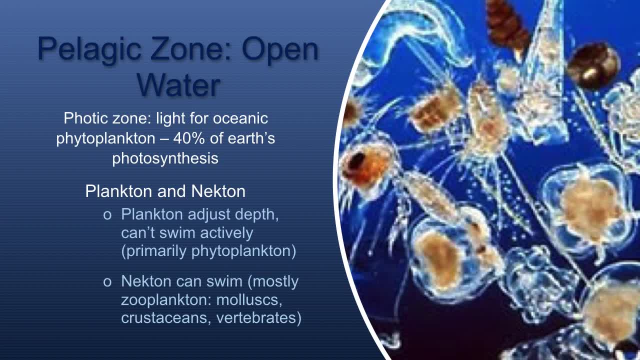 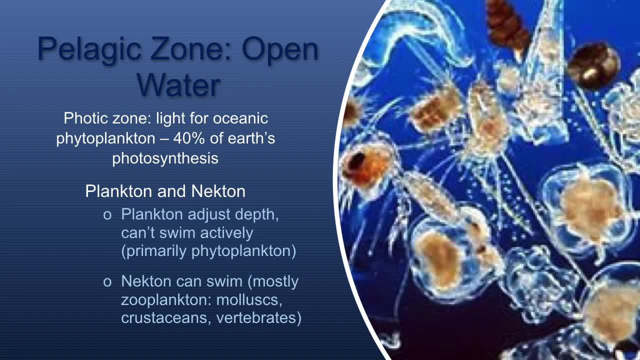 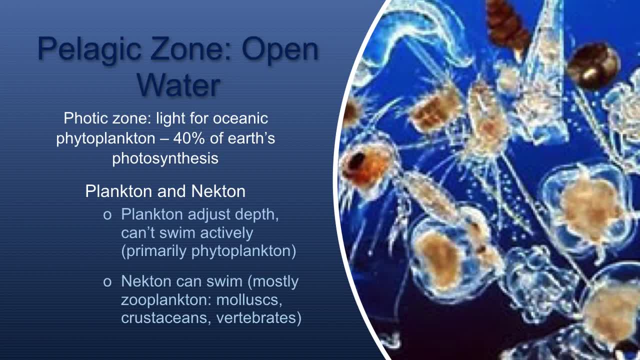 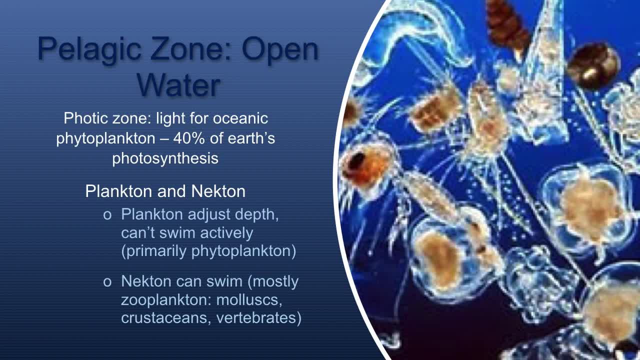 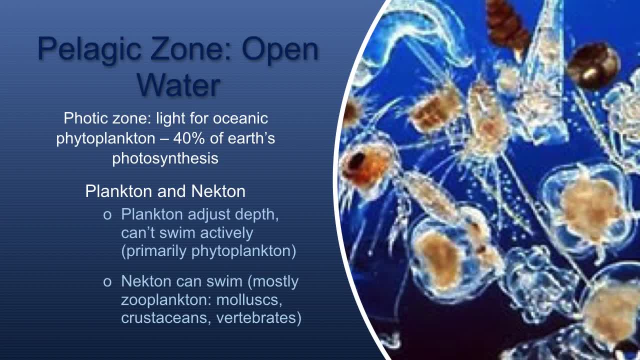 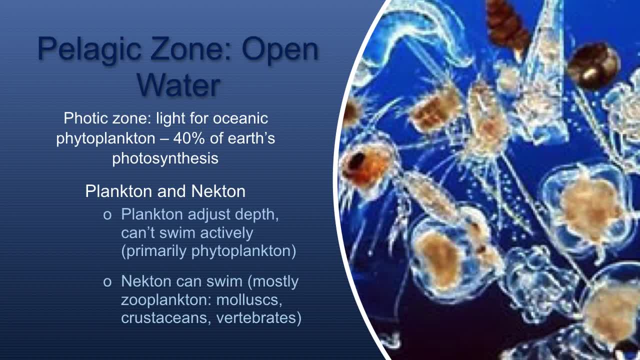 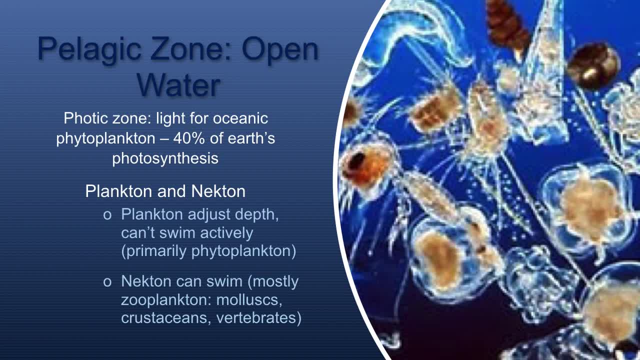 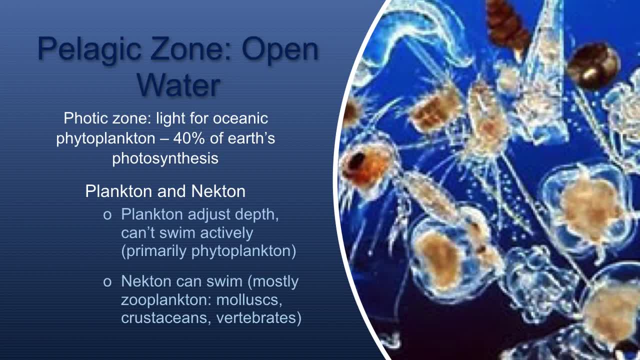 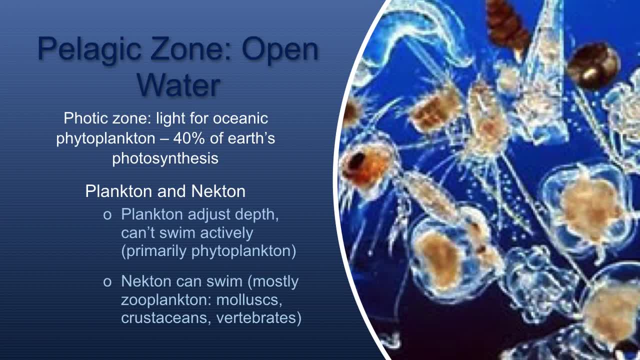 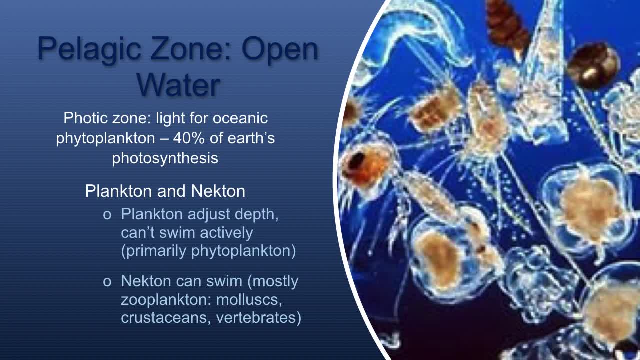 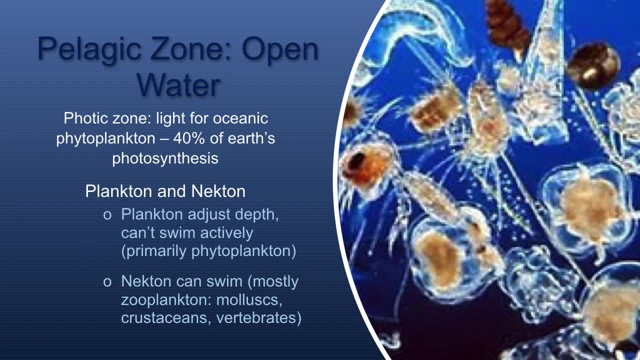 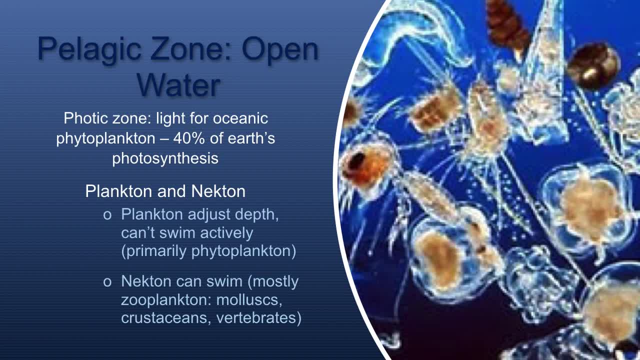 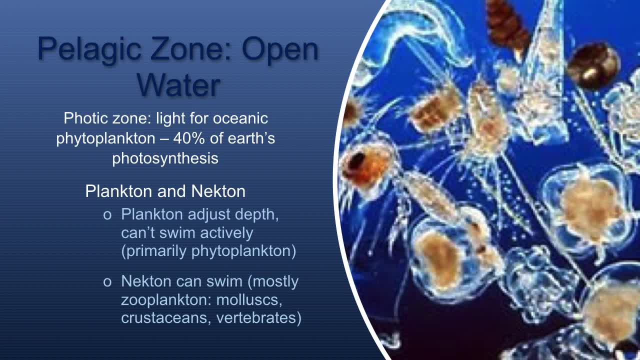 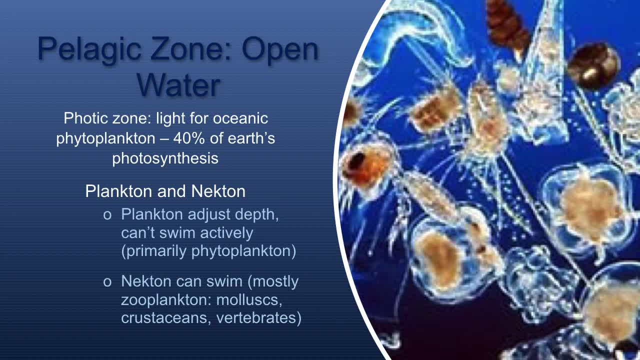 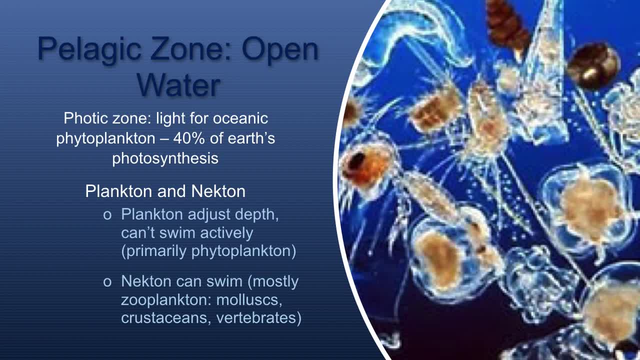 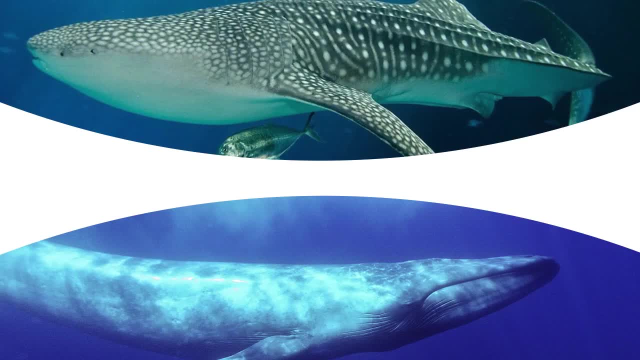 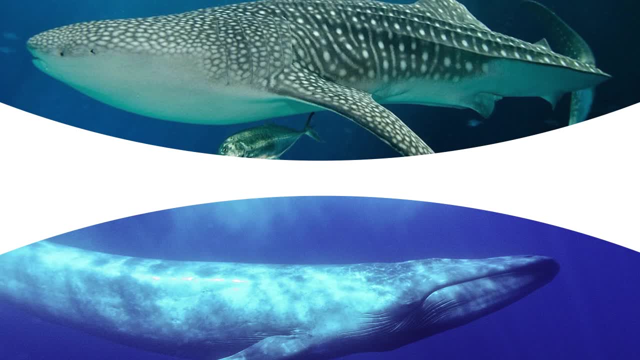 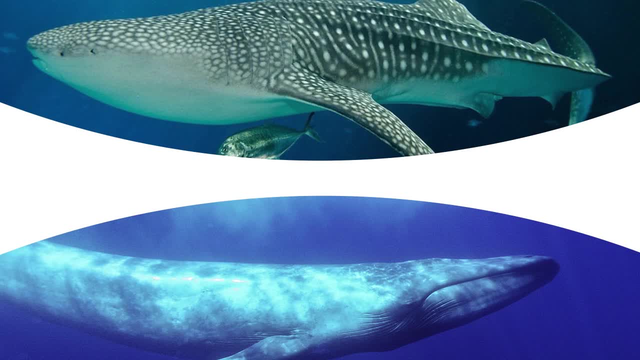 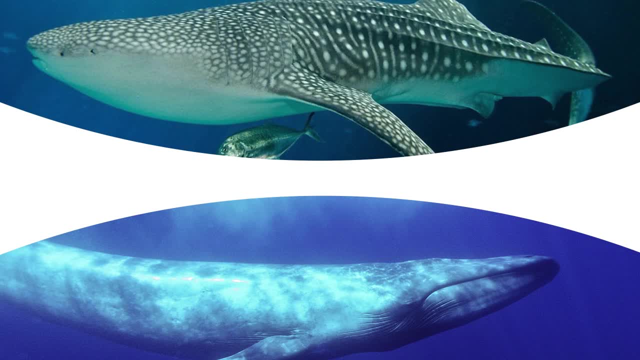 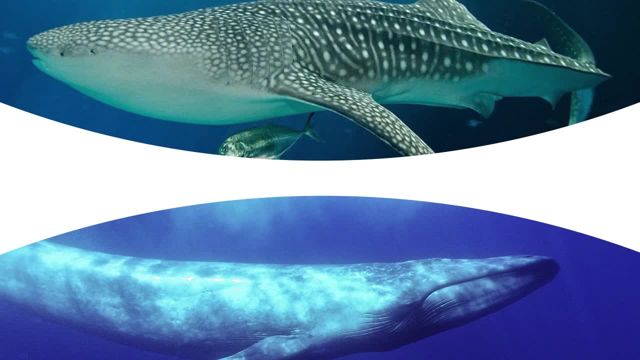 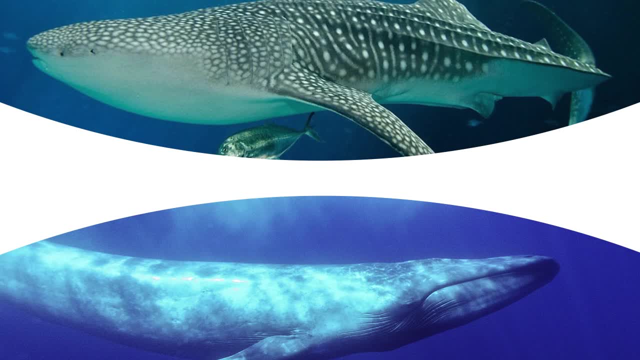 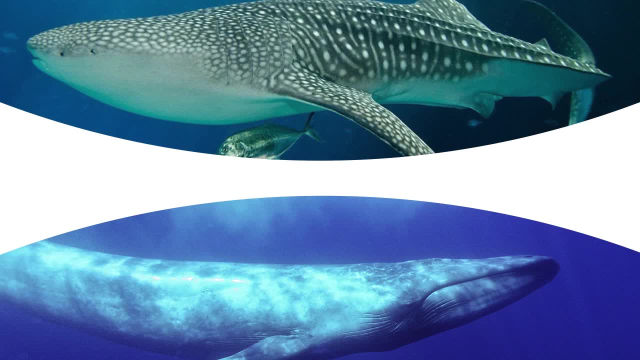 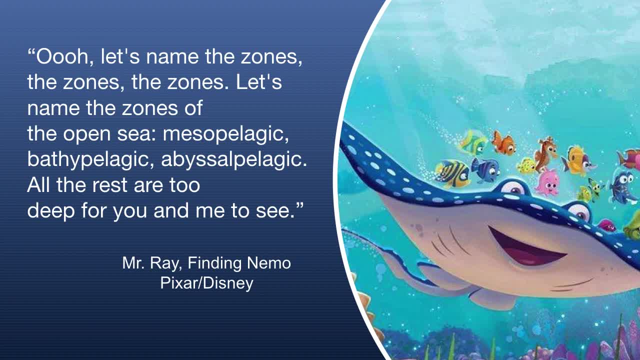 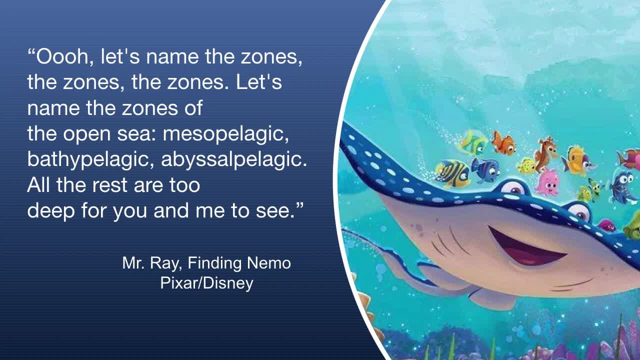 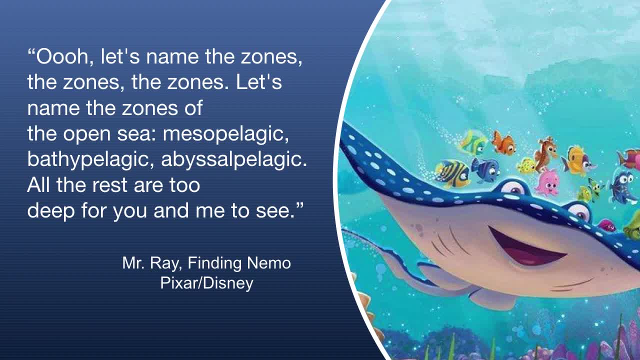 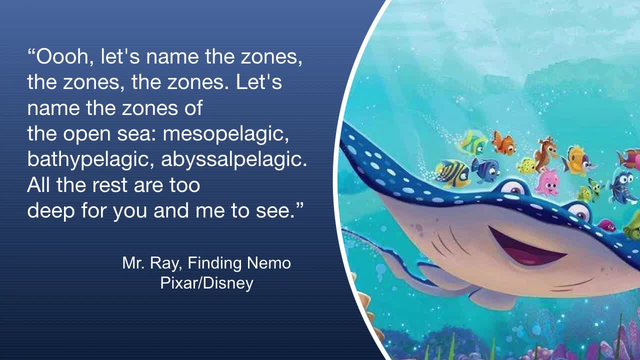 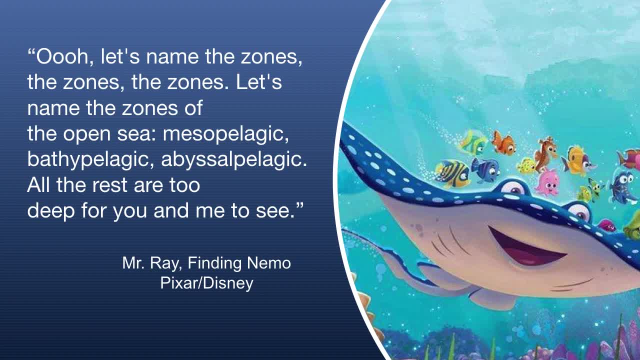 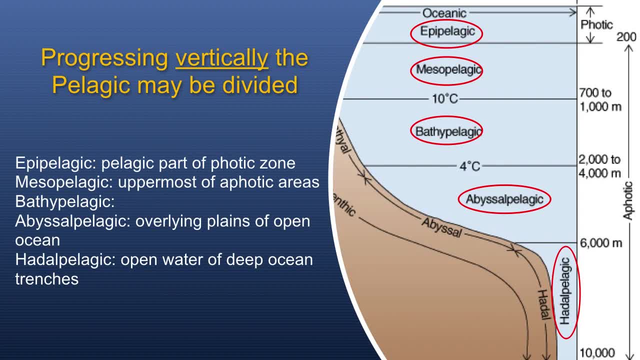 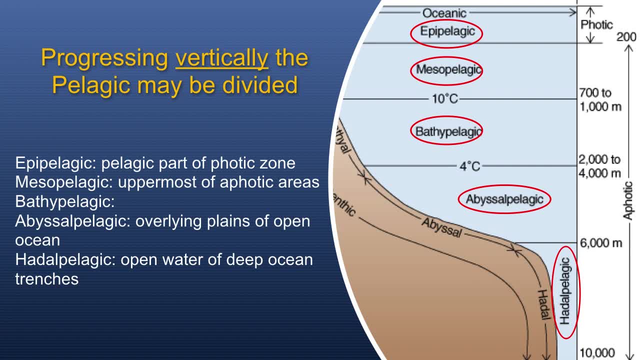 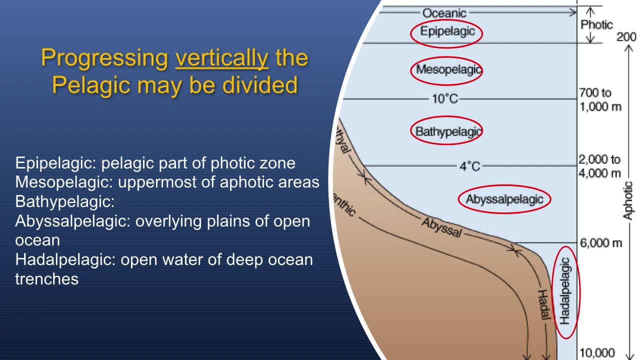 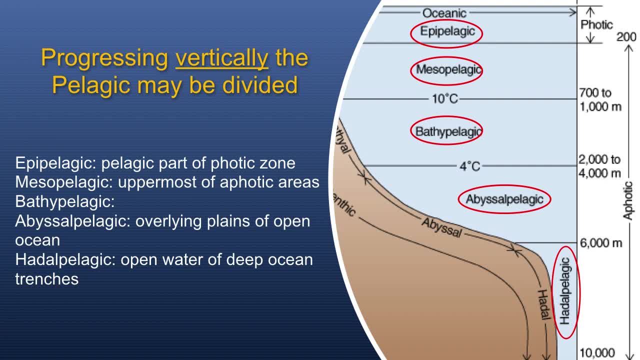 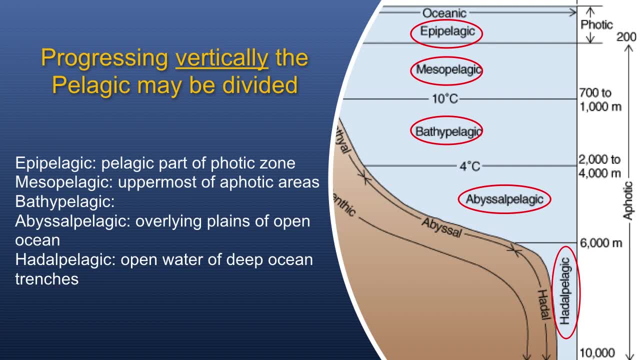 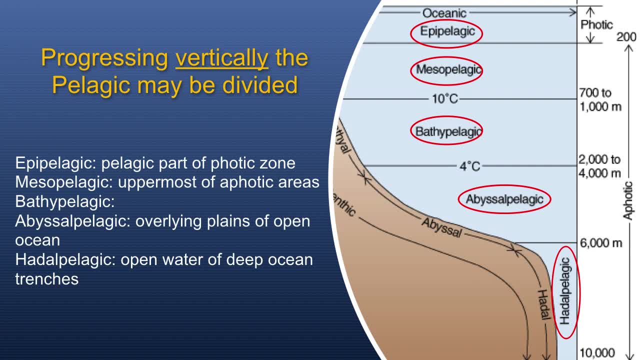 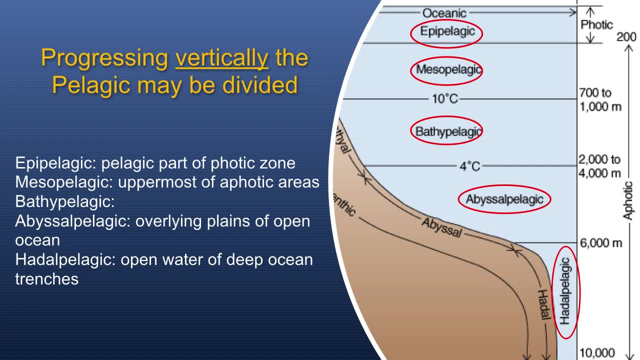 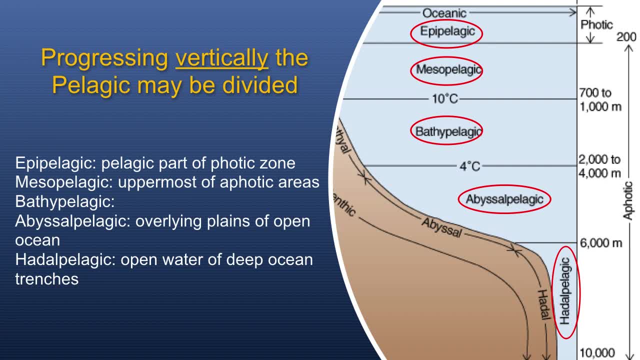 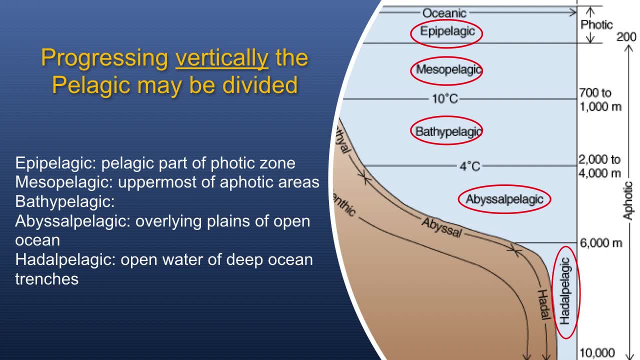 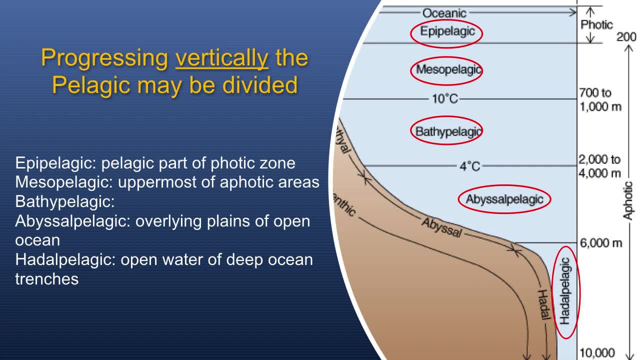 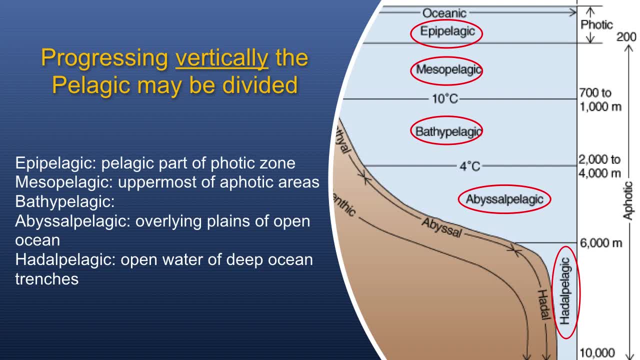 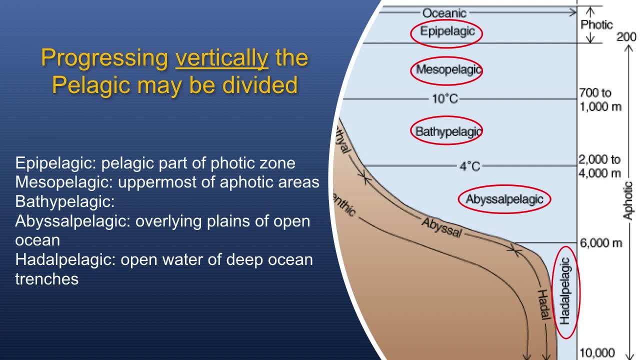 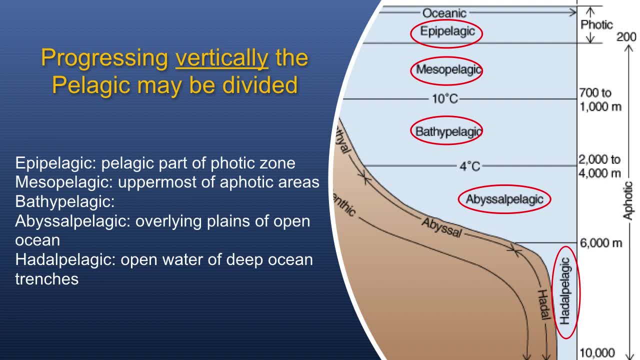 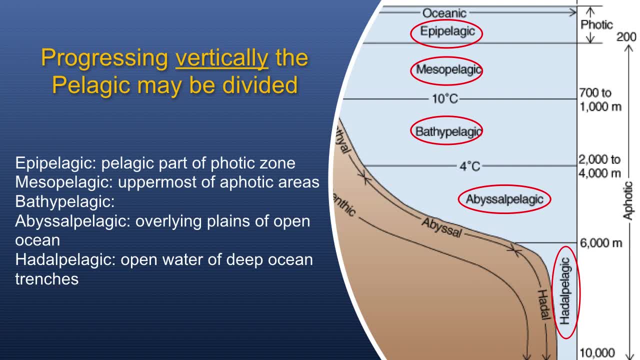 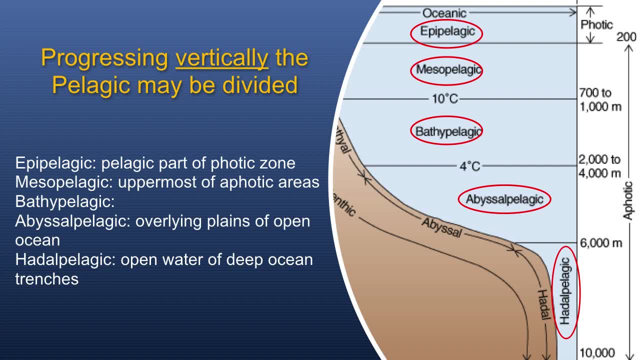 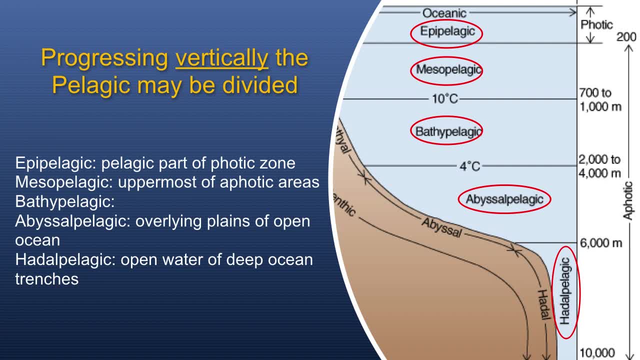 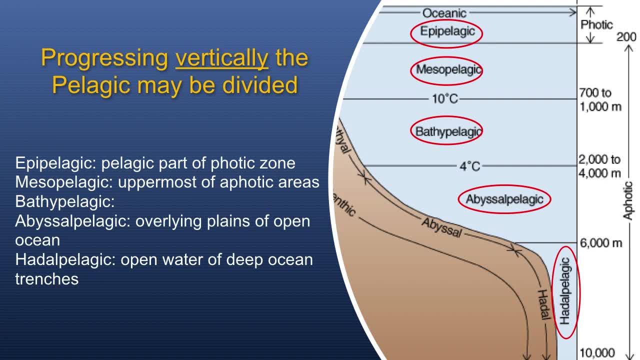 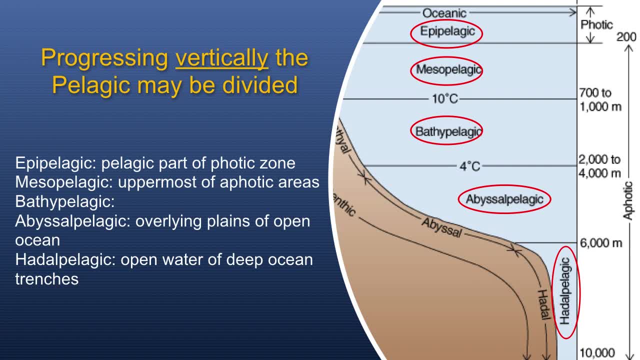 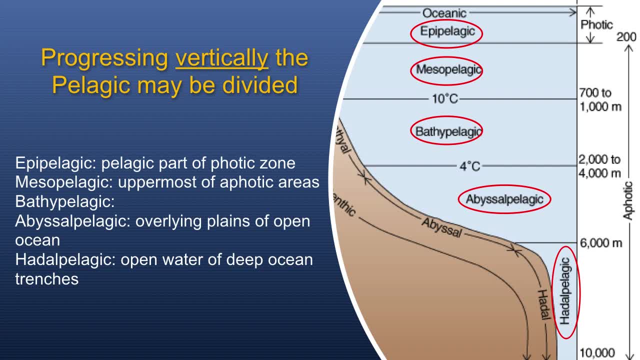 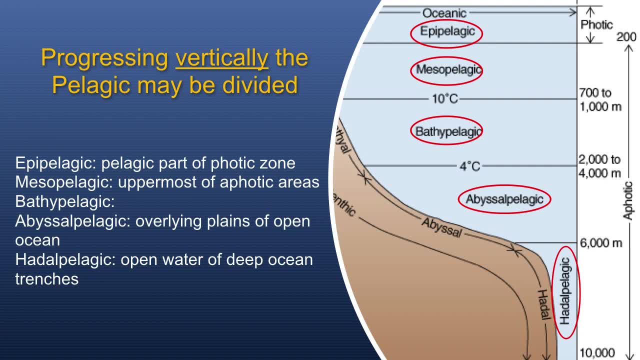 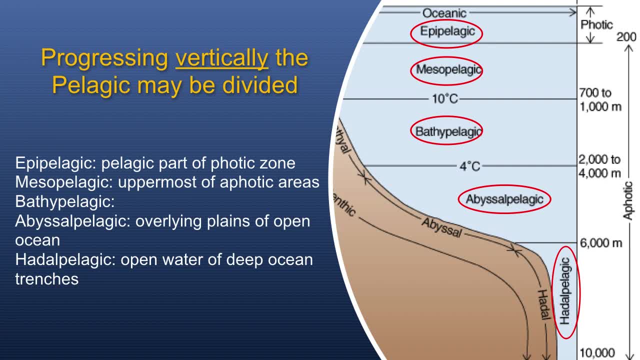 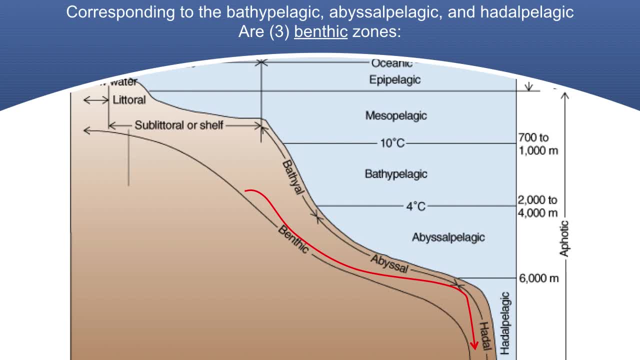 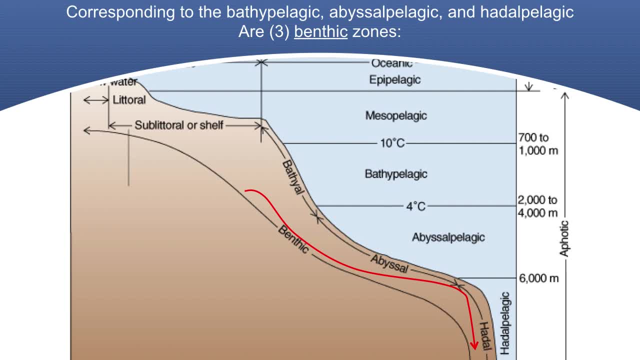 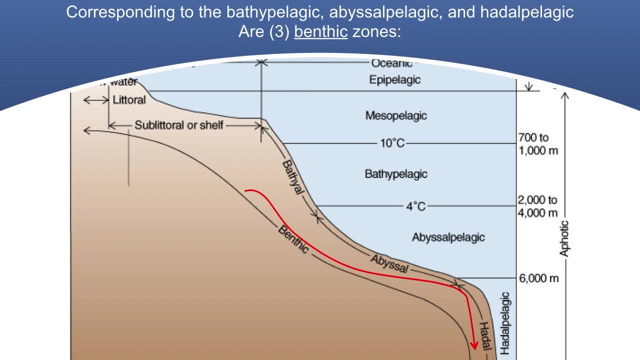 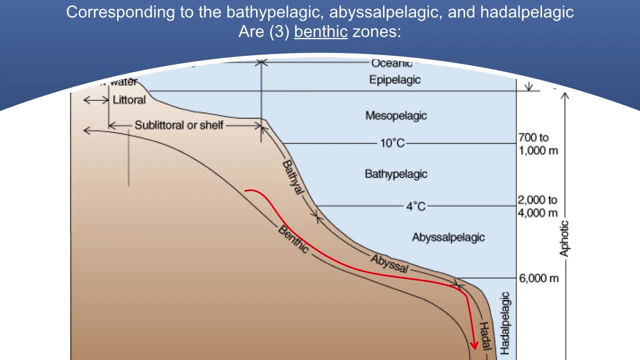 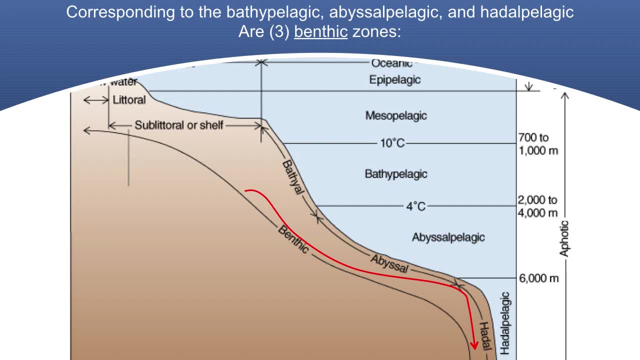 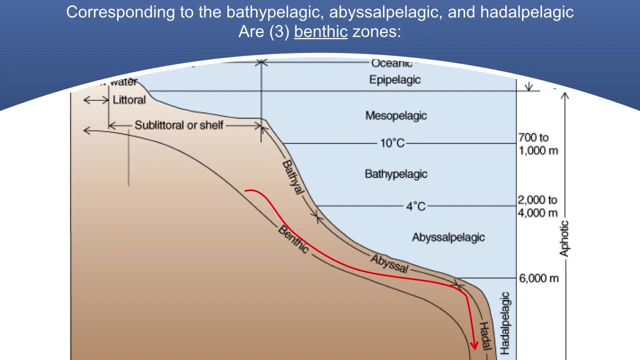 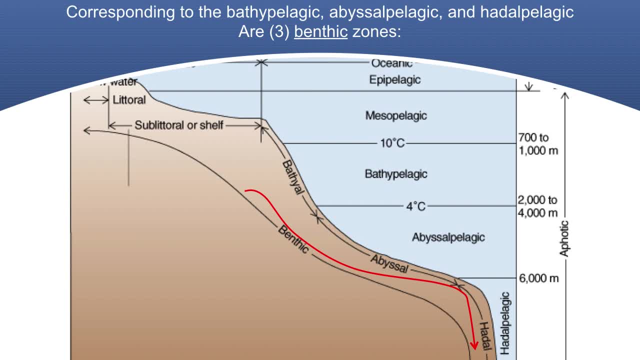 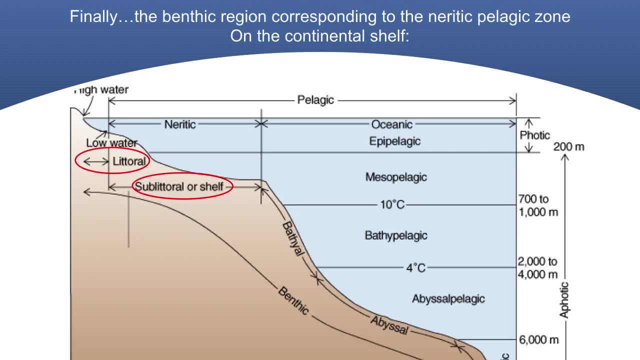 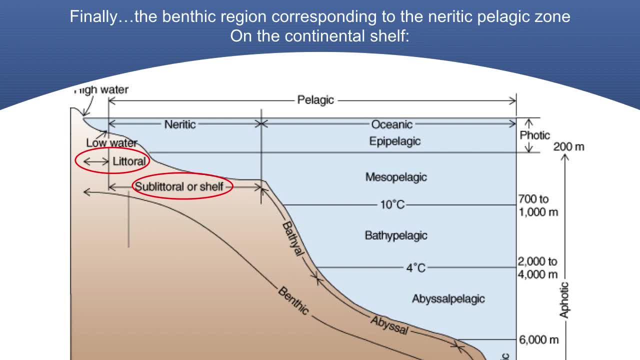 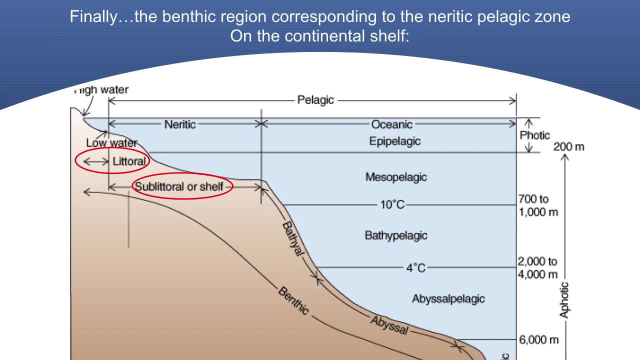 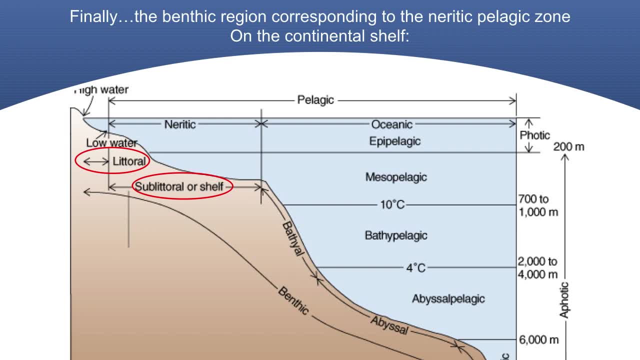 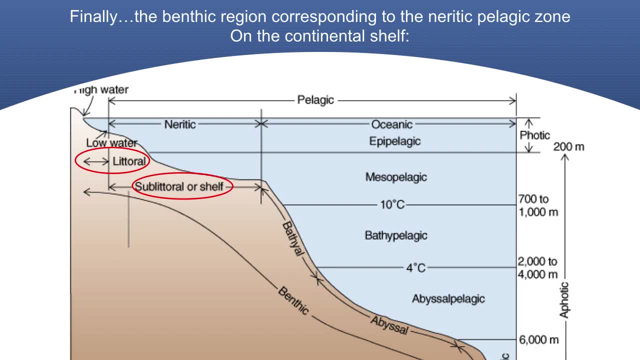 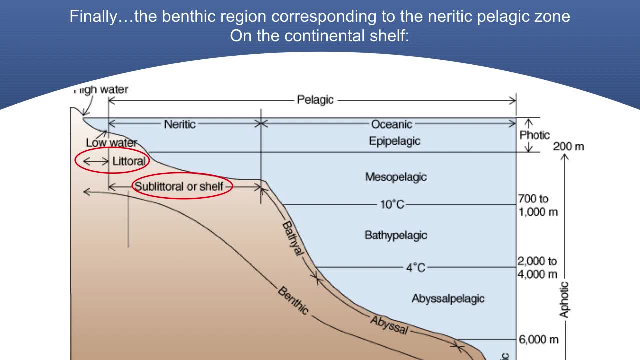 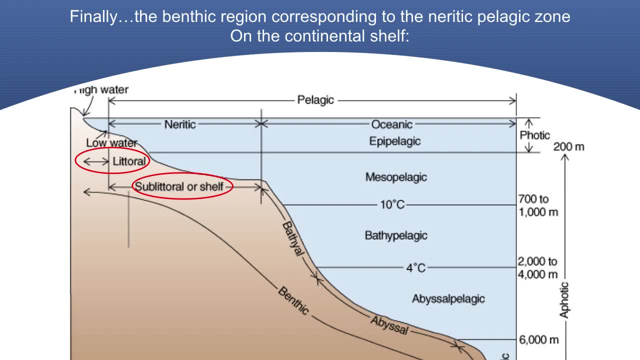 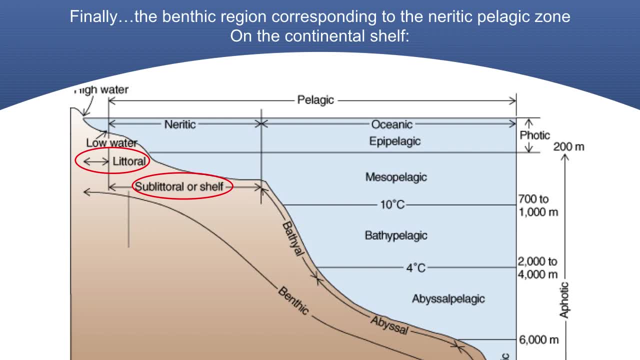 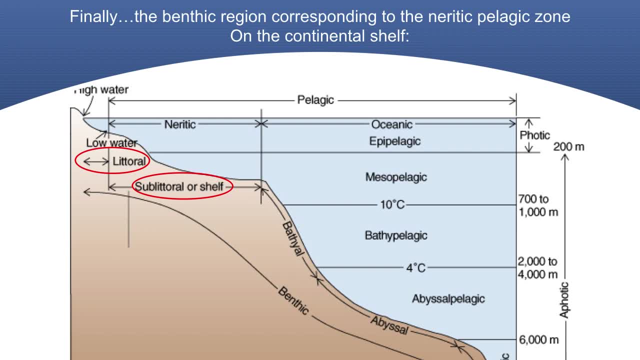 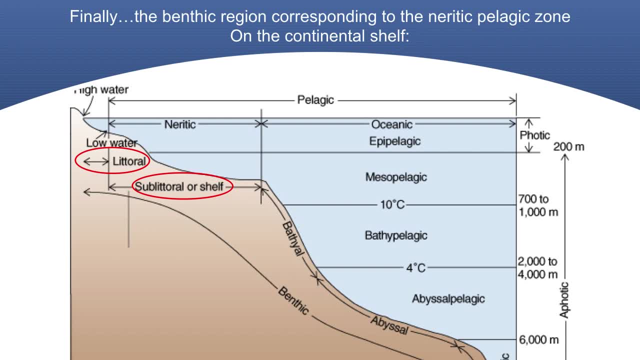 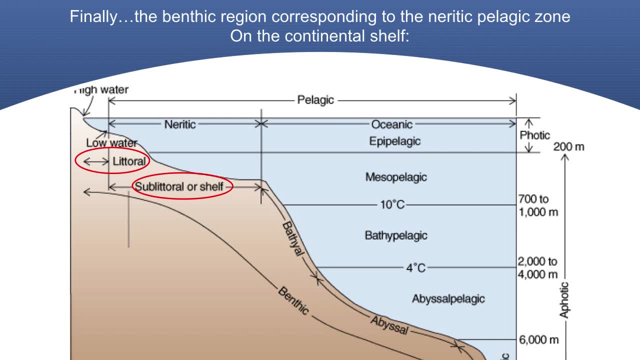 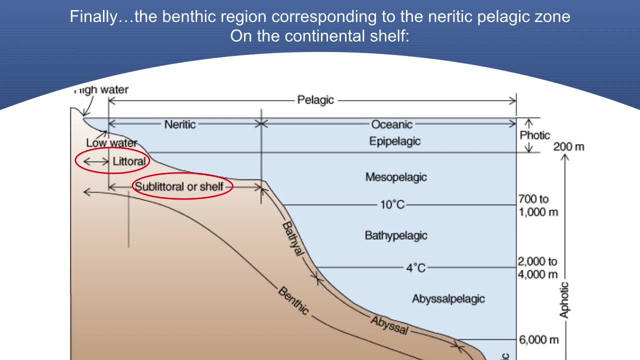 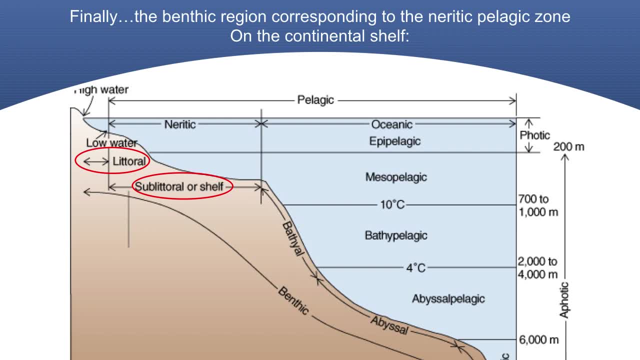 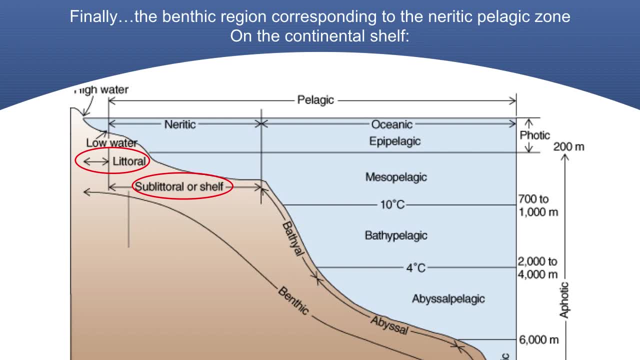 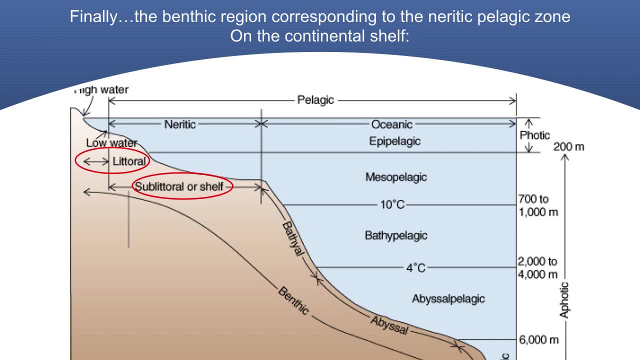 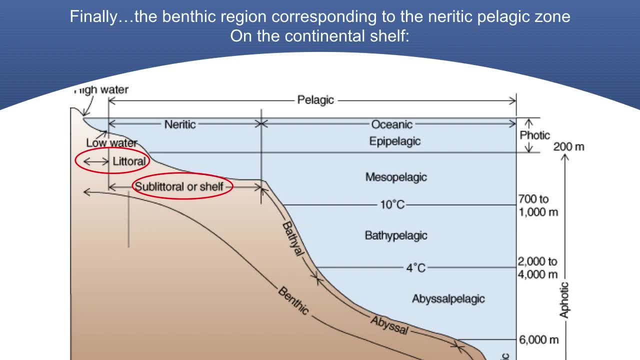 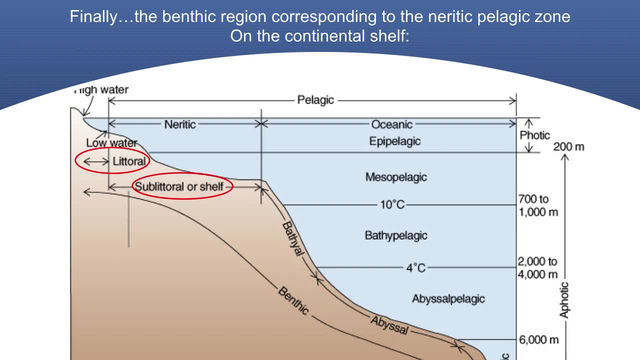 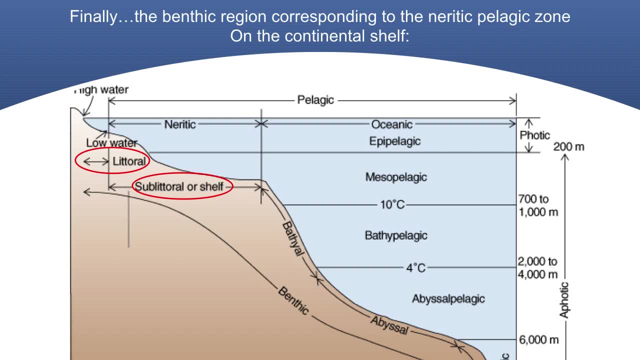 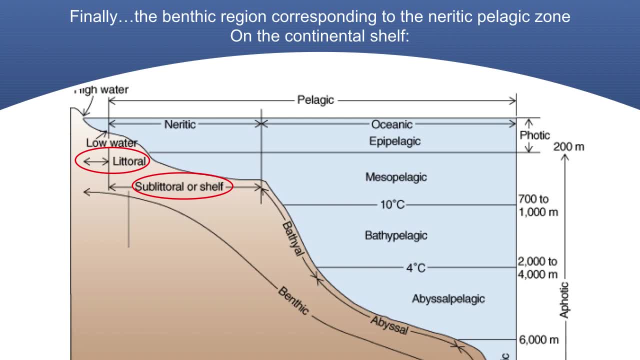 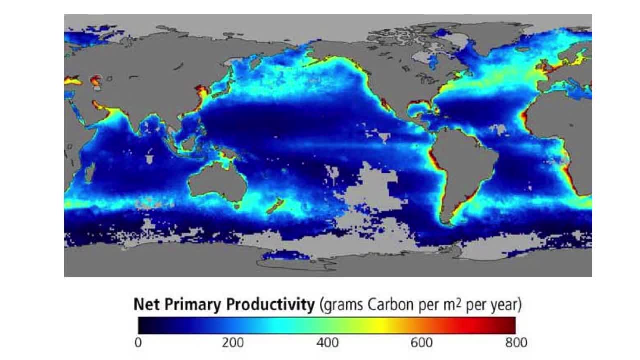 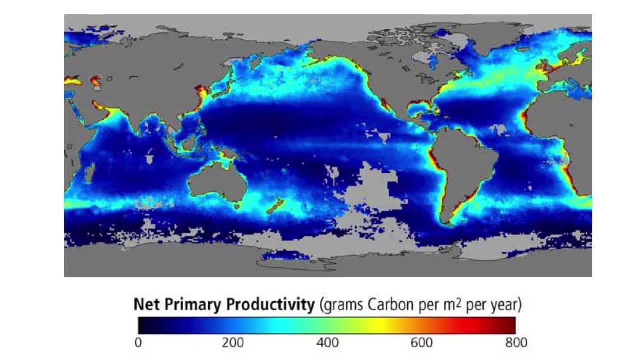 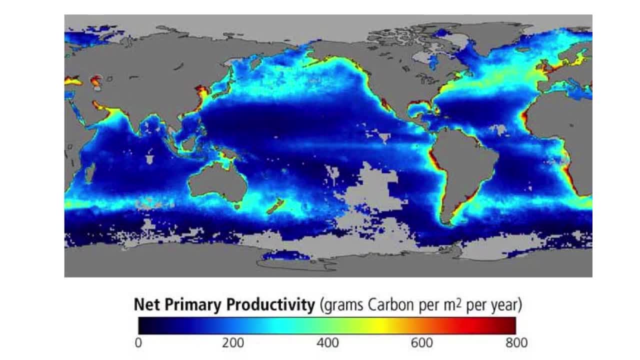 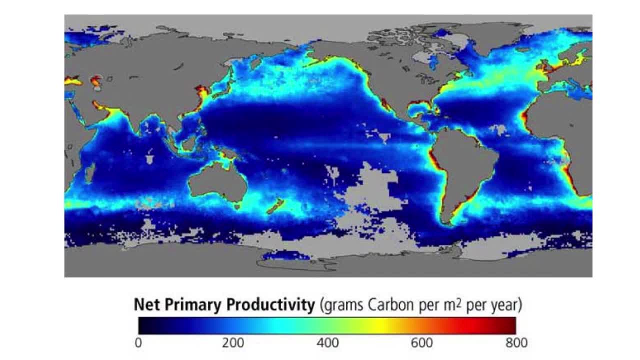 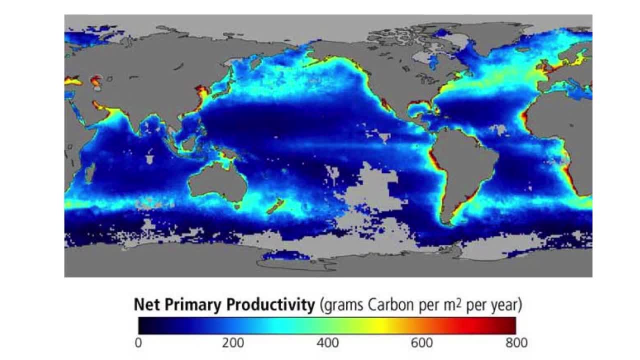 So, looking at this graph, we can see that the temperature is going up. do you think that is? We'll get to it in a future lecture, but for now we want to start our tour through the types of near shore environments and the groups of 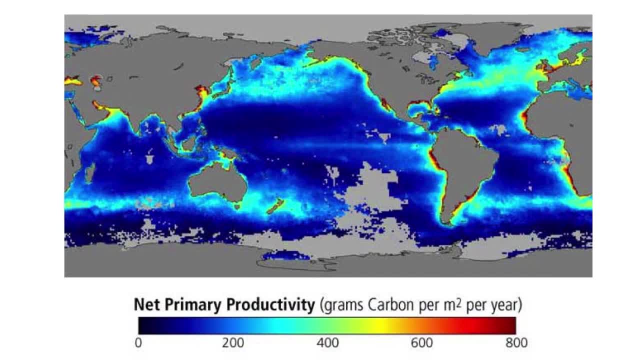 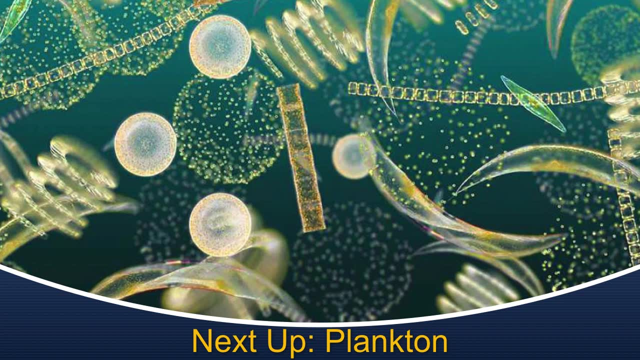 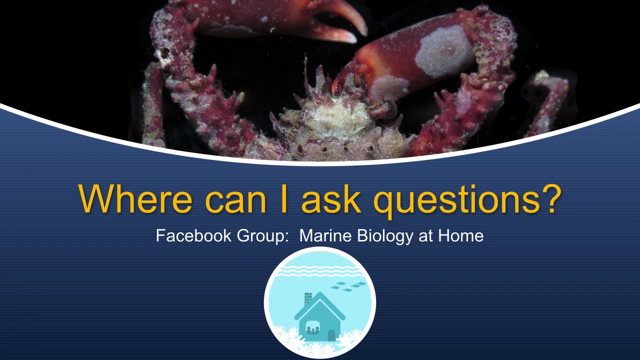 organisms found in marine systems. So what is next up? Next up is plankton. I'm excited about this one. Where can you ask questions? Well, we have a Facebook group called Marine Biology at Home that is set up for you to ask questions. So 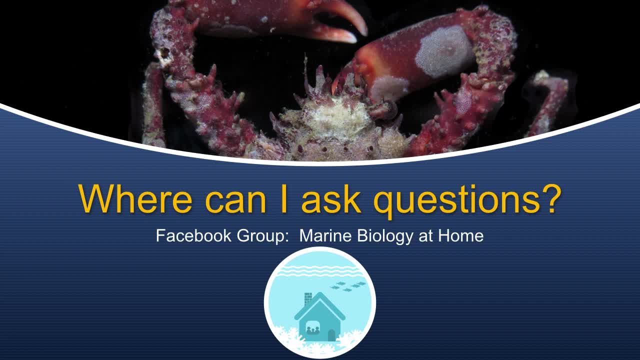 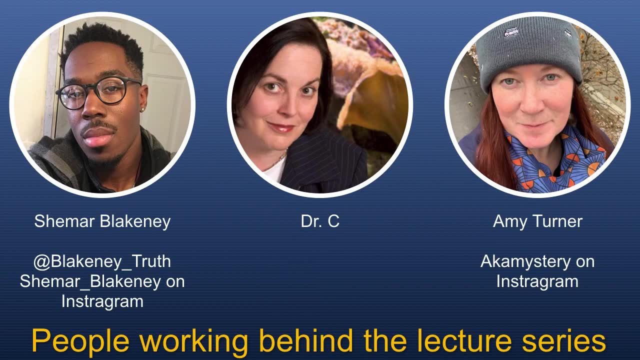 please take advantage of it. We have lots of expert folks standing by, some of which are great people like Shamar Blakeney, and you can find Shamar at at Blakeney underscore truth or Shamar underscore Blakeney on Instagram. Dr C- the famous Dr C. 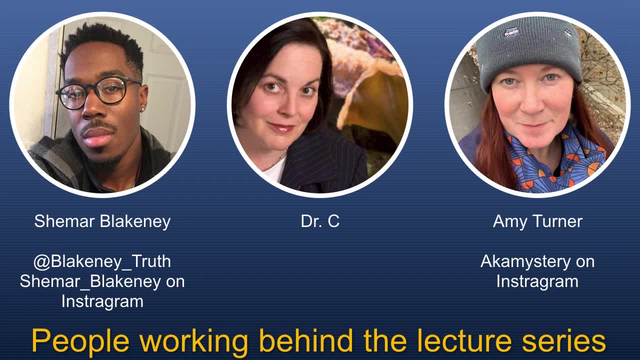 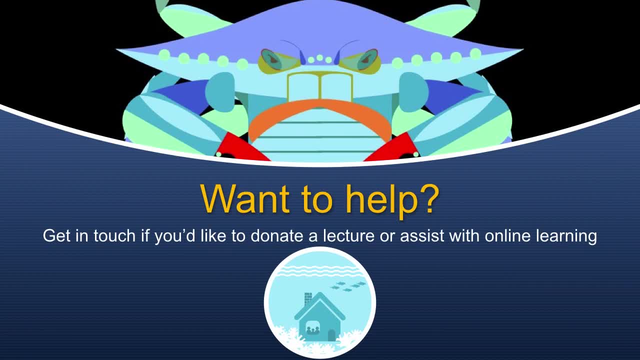 series that hopefully you will see more of coming up. If you would like to help, please get in touch. If you would like to donate a lecture, if you are a marine scientist or a marine educator, or if you'd like to assist with online learning. 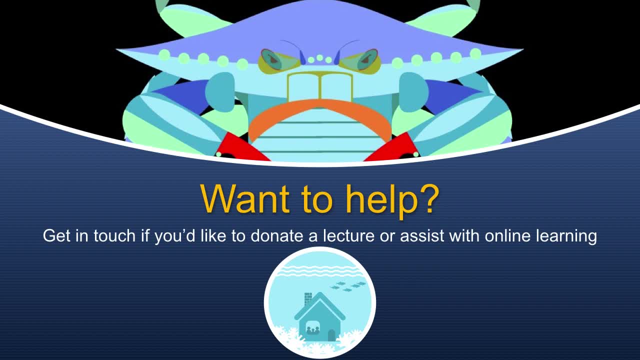 as a student or someone who's still actively studying. we would love it, So please reach out. We will see you soon.